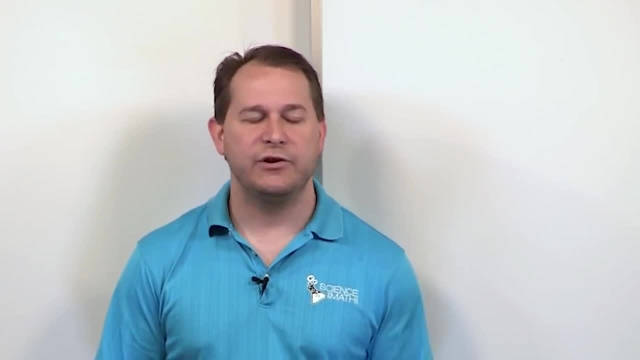 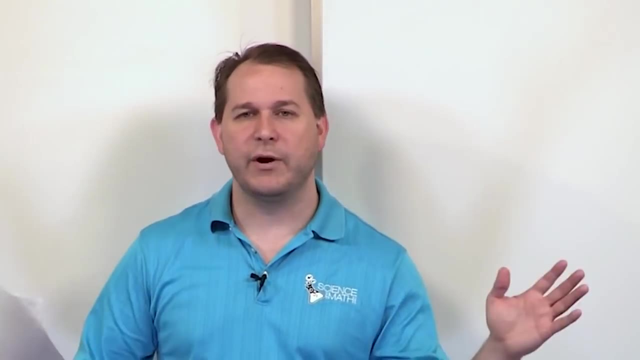 of books are super hard to understand with what these things really mean And you look at equations and formulas and lots of drawings and then you can just go nuts. I'm going to make it very, very easy for you to understand. Just take a deep breath, realize that this. 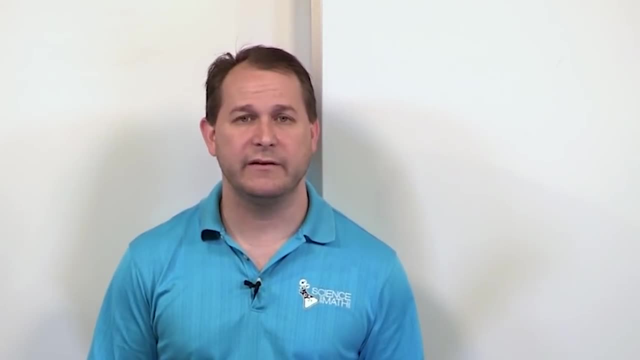 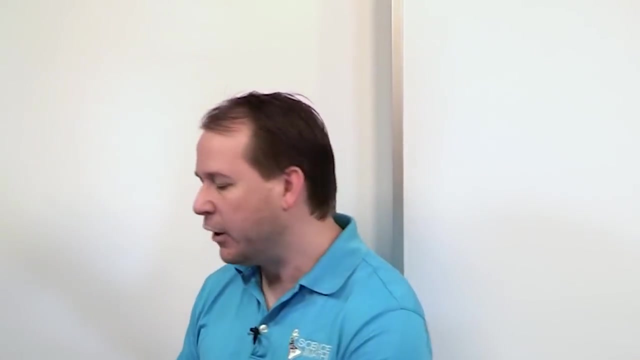 is very simple. By the end of this lesson, you'll know exactly what a probability distribution is, what makes it discrete, what a random variable is and how it is different from a regular variable in algebra. So we need to go through some definitions. We are going. 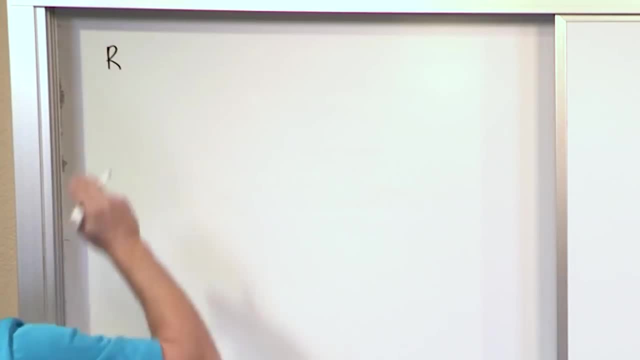 to take a little bit of time. We're going to take a little bit of time to go through some definitions. We are going to take a little bit of time to go through some definitions, So let me write them down and then I promise I will make sure that everything is absolutely. 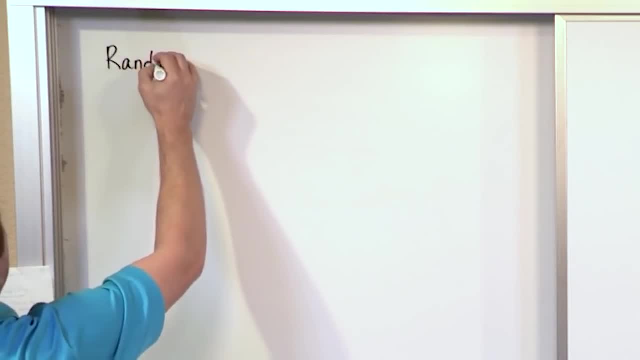 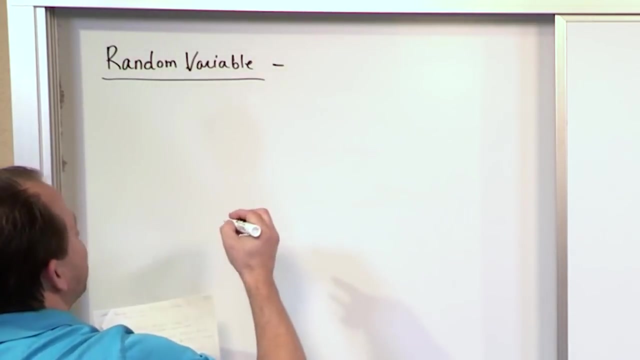 clear by examples. So here we have the idea of a random variable. In algebra, a variable is just something that can change or take on different values. Variable- the word variable means that it can change, But in statistics a random variable is a variable whose value. 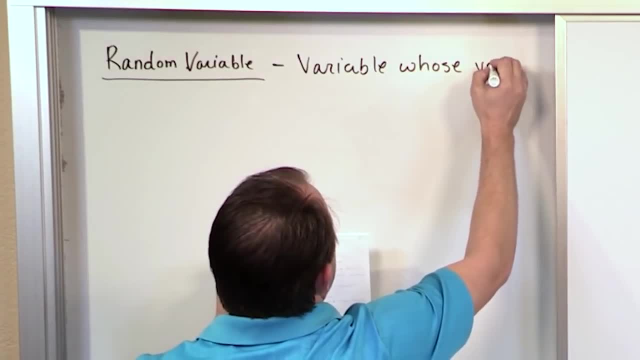 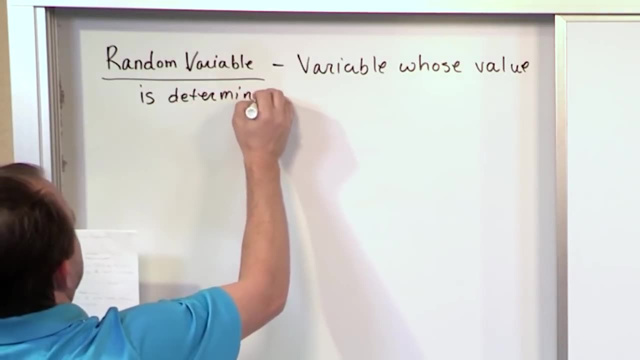 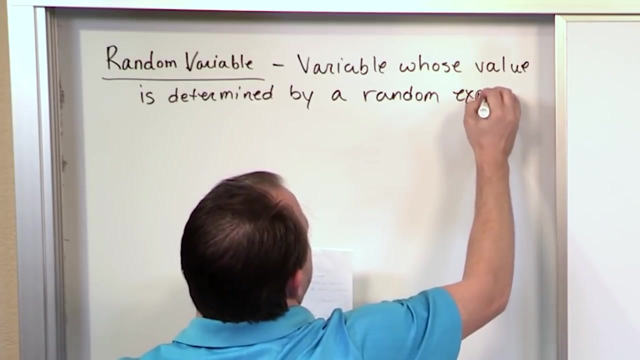 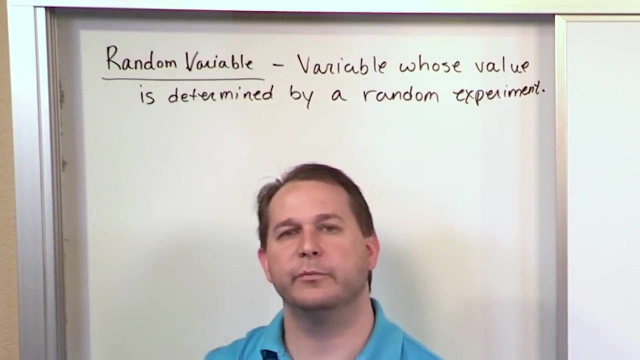 is determined by a random experiment. And when we say experiment in the context of statistics, I'm not talking about beakers and test tubes, I'm talking about you. do something like An experiment might be drawing two cards from a deck of cards or something, And then you 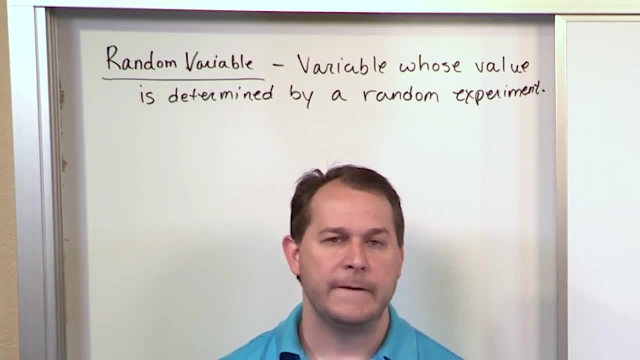 can do everything. You can draw the answer to the question and then you can do something. OK, So what you'll do: first you're going to draw the answer to the question And then cards. What's the chances that I'm going to get two aces or two fours or whatever There's? 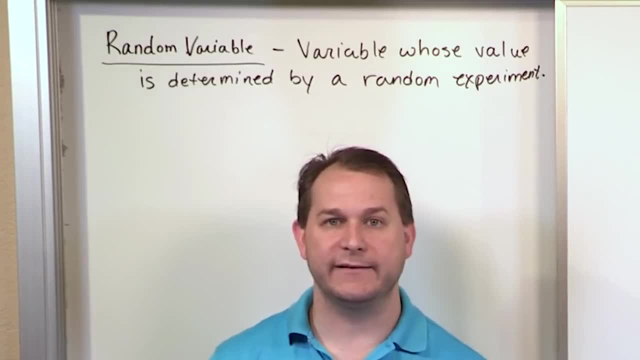 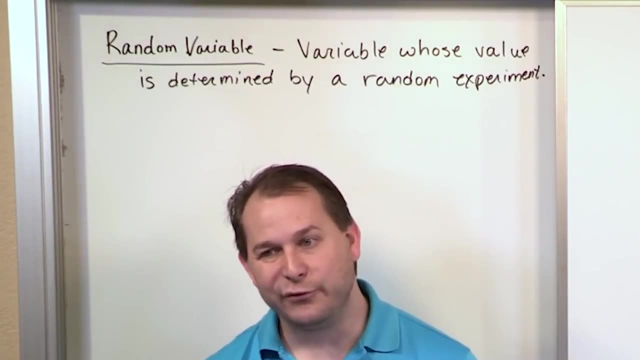 a way to calculate that. Now, if I repeat that experiment with new decks, you know, or maybe I shuffle the cards back into the deck to make a complete deck, I can do the experiment again. Well, did I get two fours that time? No, Okay, I can put it back in. 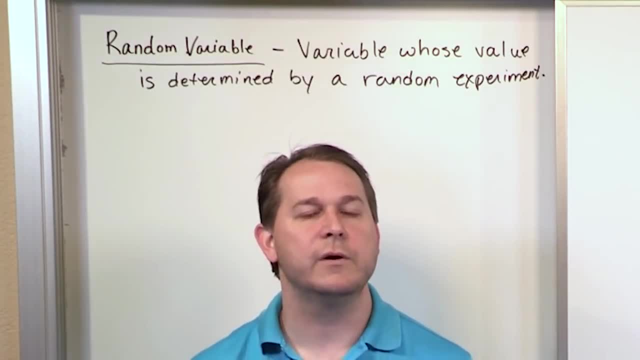 do it again. Well, eventually I'm going to hit two fours. Eventually, if I do the experiment enough, I have a deck of cards and I draw two cards at a time. eventually I'm going to get two fours. It may not be on the first try, it may not be on the tenth try, it may. 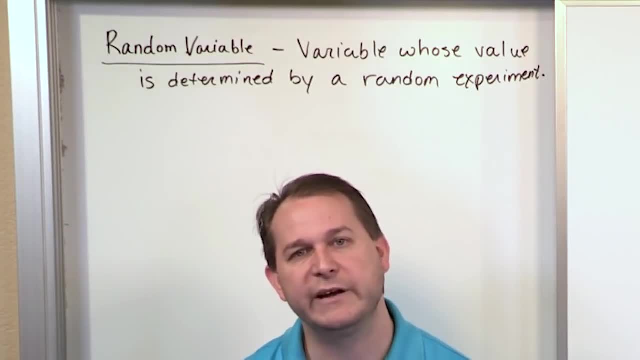 take me fifty-five tries or two hundred tries, but eventually it will happen. So when I say random variable, it doesn't really mean that it's randomized like a random number generator. It just means that the outcome of the experiment is basically going to be. 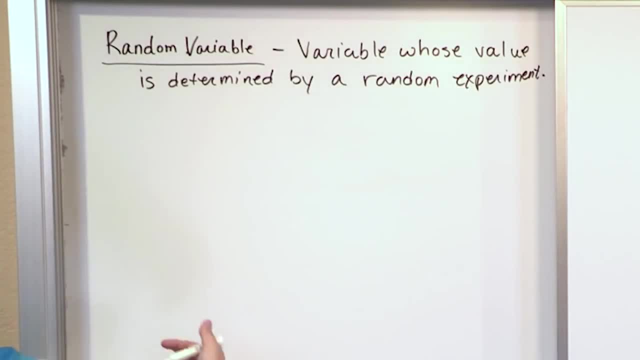 assigned to a variable. So the variable in this case could be: what do I do? what do I get when I pull two cards from the deck? Well, the value of that variable, or the outcome of that variable, is determined by a random experiment or some kind of statistical. 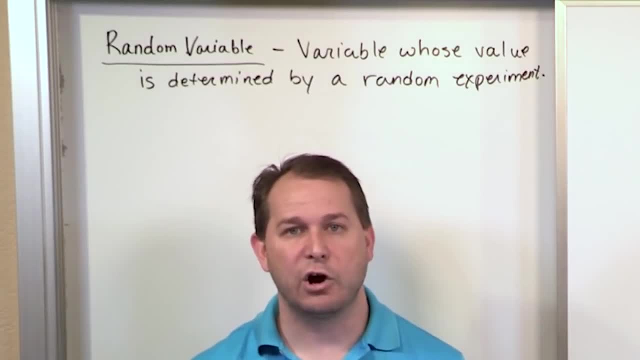 process. It could be flipping coins, it could be pulling stuff from a deck of cards, it could be observing population and asking a survey or something. It could be lots of different things. A random variable is just the outcome of an experiment and you do the experiment. 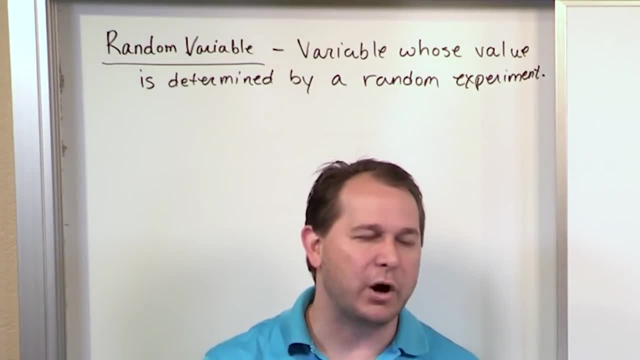 a bunch of different times and you get a bunch of different outcomes. So the random part just means that you're doing it over and over again. You don't really know what's going to happen ahead of time, Unlike in calculus or in algebra. when you solve for a variable, the variable is always going to be, you know. 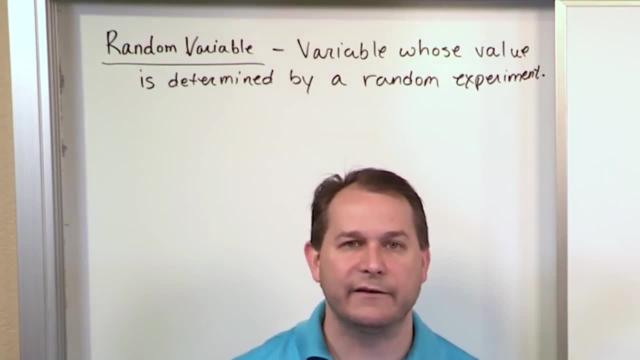 if you have a simple algebra equation, you can solve that equation and you get an answer. The answer might be two: right, That's the variable. you solve for the variable. That's the answer. But in statistics the variable really depends on the experiment. and if I 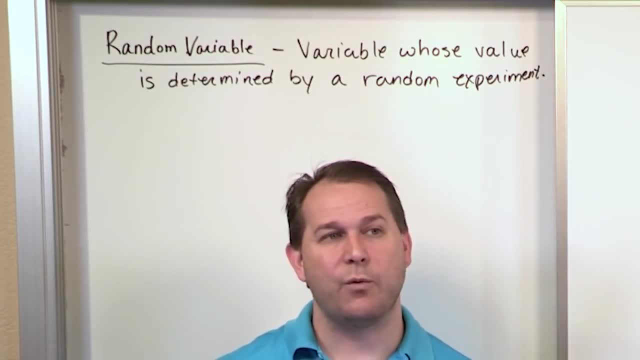 do the experiment four times, I might get different answers. okay, Now what I'm interested in in statistics is what happens if I do the experiment a thousand times. Can I draw conclusions? Is the random variable going to take on some values more likely than others? 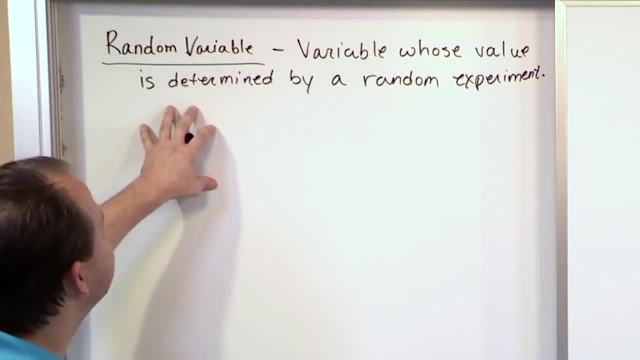 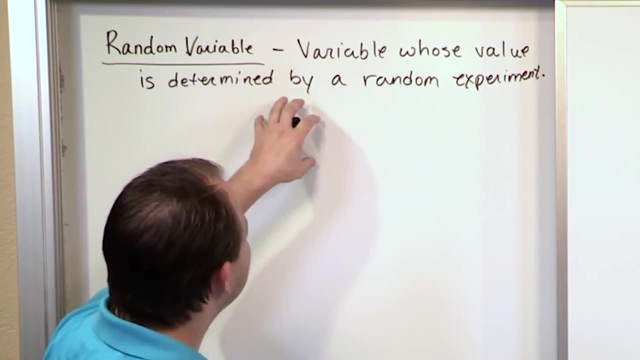 If I do this experiment a lot of times. But anyway, the concept of the random variable is just: I do an experiment and then I do it again, and then I do it again, and then I do it again Each time I get a result. usually I'm looking to see the specific outcome of 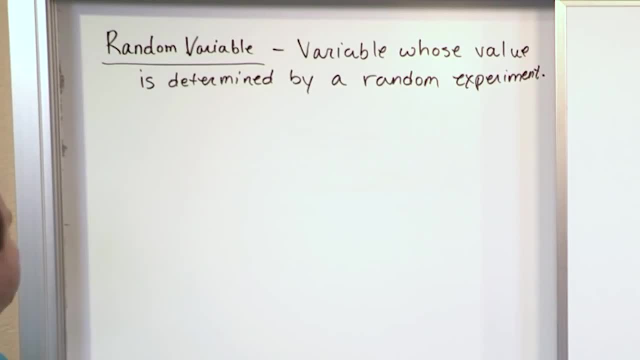 something and we're calling that a random variable because it might change each time I do the experiment Now. I'll give you some more concrete examples in a minute. Let me show you what the idea of a discrete probability For probability. I'll just do prob like that. 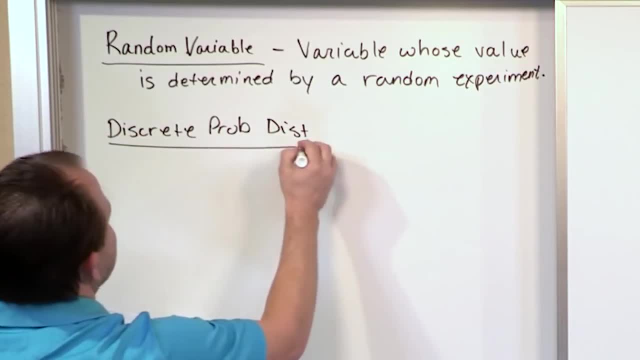 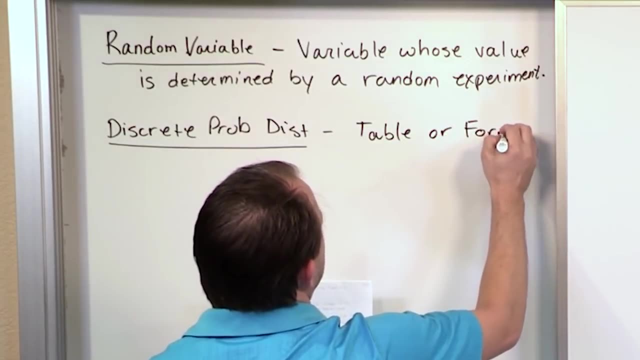 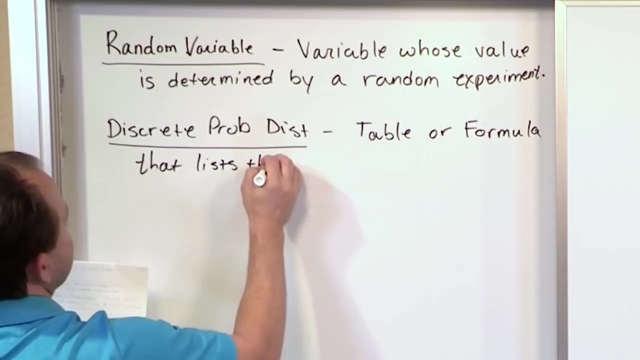 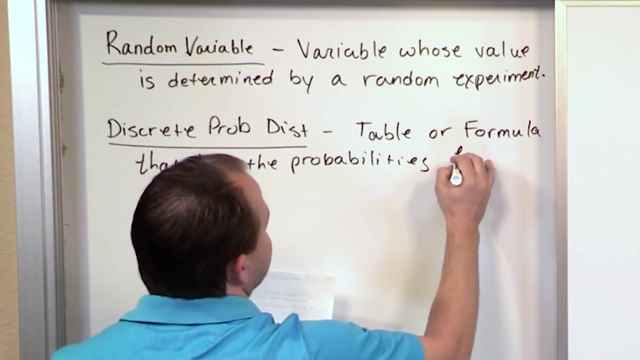 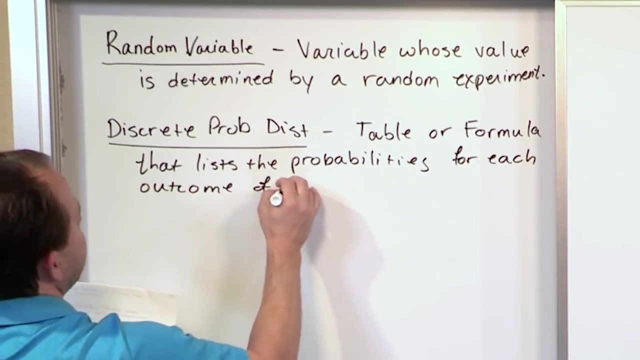 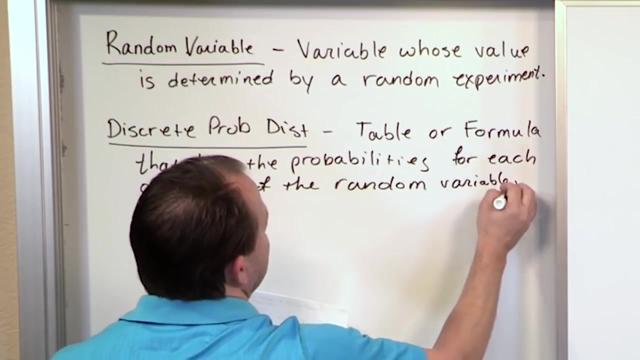 And for distribution I'll do dist like that. So this is discrete probability distribution. It is a table or a formula that lists the probabilities for each outcome of the random variable x. Now notice also the random variable we're calling x Usually. 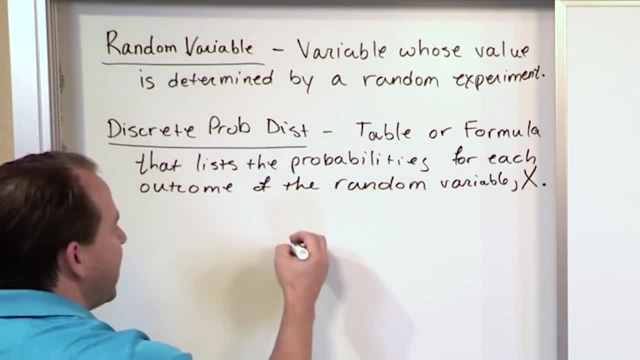 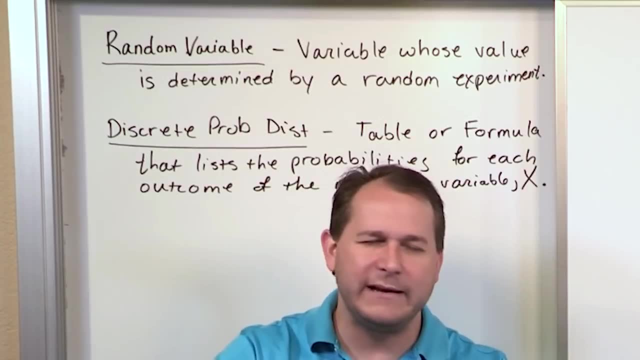 in statistics it's a capital X. Usually you know, in algebra you have a little x, or you could use y or z in algebra, But in statistics when it's a random variable, which just means it's an outcome of an experiment, that's all that. a random variable is you. 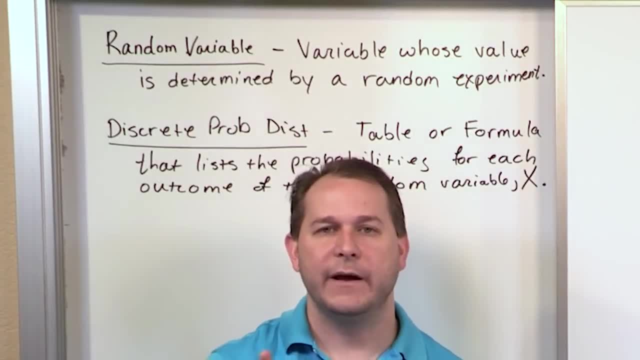 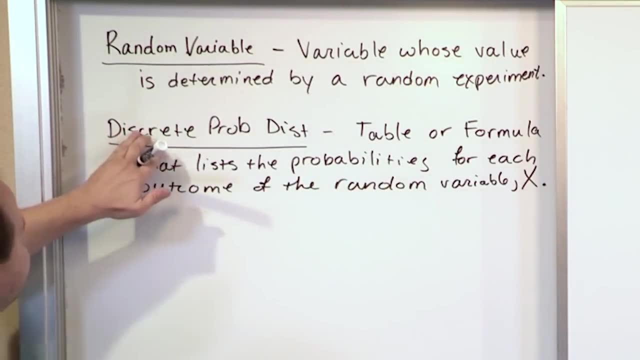 use a capital X, No curvy x's or anything like that. That's for algebra or calculus. In statistics we use capital X. That means random variable. So don't worry about the word discrete, I will explain that in a minute. But the probability 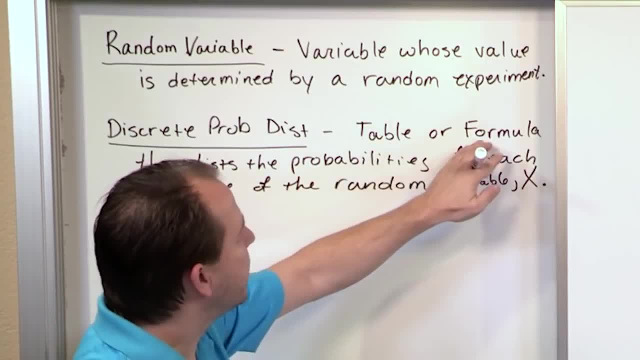 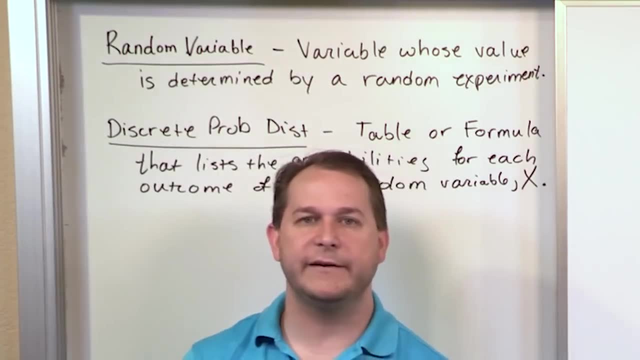 distribution focused on that. it's a table or a formula that lists the probabilities for each outcome of the random variable x. So, as we talked about with the idea of shuffling a deck of cards, we're going to get different outcomes when we draw two cards. We're going 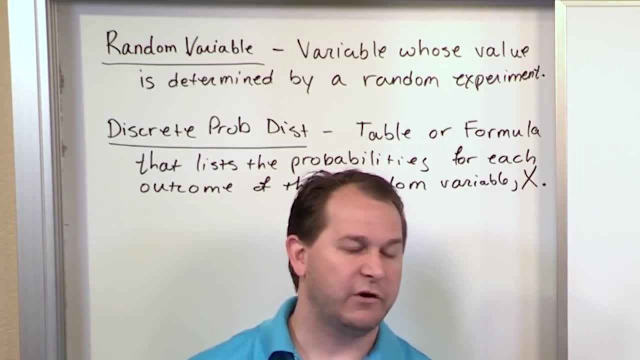 to get different outcomes. Now. sometimes we might get totaling, Sometimes we might get two, you know, a pair. We might get a pair, which means two cards of the same value. right Now. there may be different probabilities associated with all. 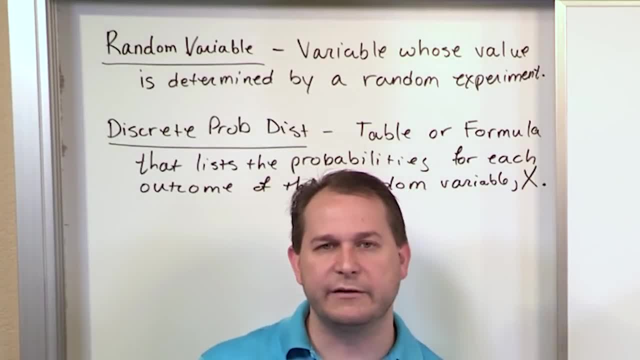 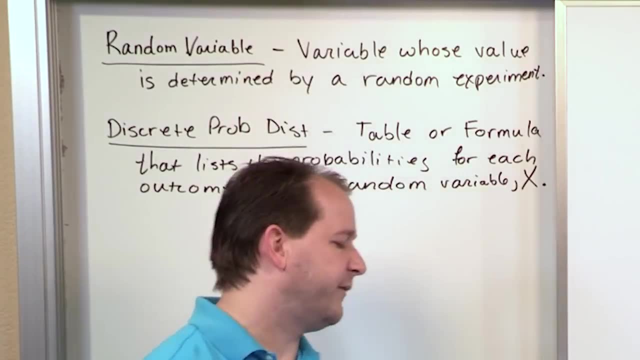 those different outcomes And the distribution of what those probabilities are is what we're talking about. It's called the probability distribution. Most of the time it's represented as a table in terms of the discrete probability distribution. here Again, I'll talk about 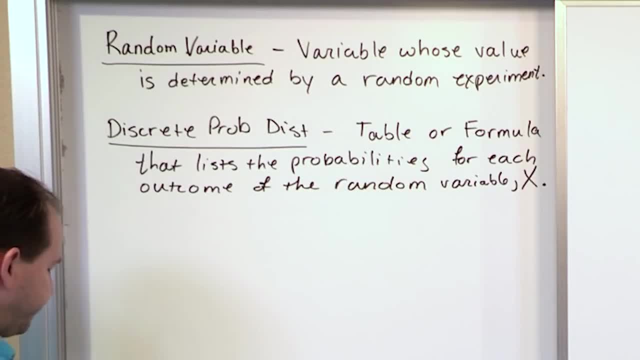 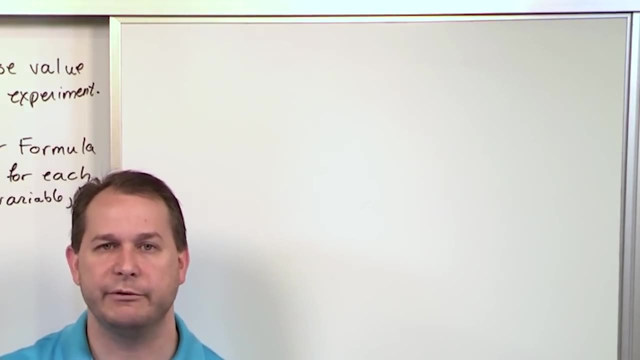 the idea of the discrete in a second. So for a concrete example, I hate just putting something on the screen forever like this. What I want to do now is I want to give you a real example and show you what a distribution, a probability distribution- 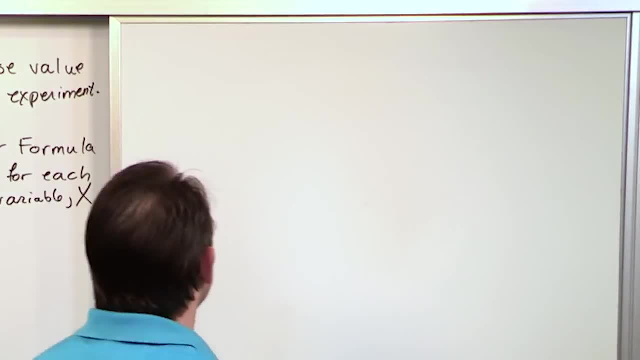 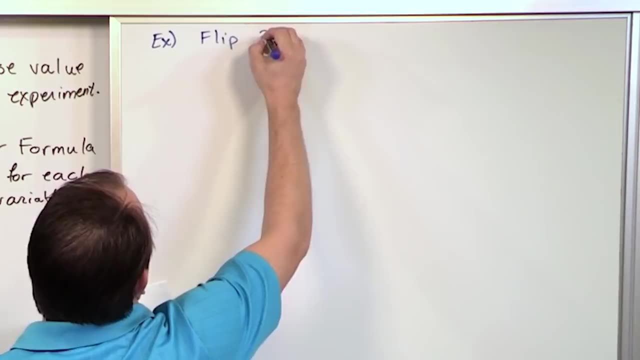 is. It's going to be much more concrete than a bunch of words like this. So for an example of a discrete probability distribution, let's say: let's flip three coins, So we're not just flipping a quarter, We're flipping three quarters at the same time. 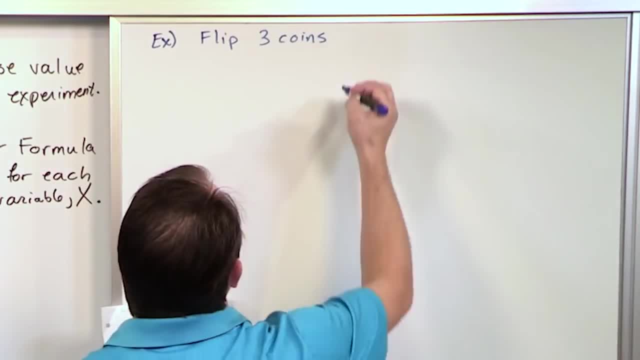 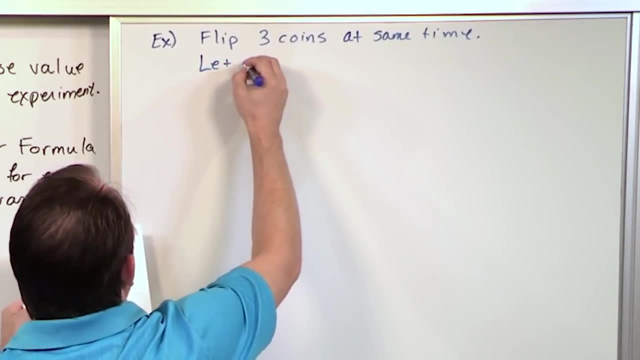 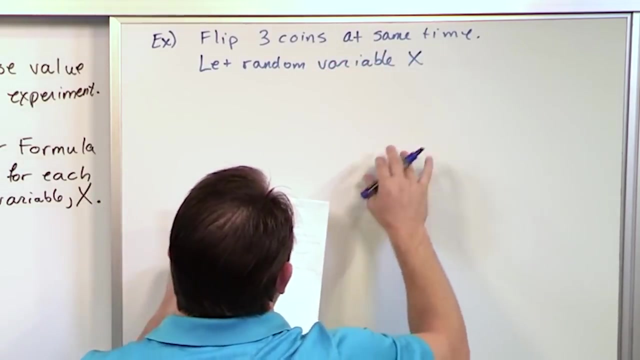 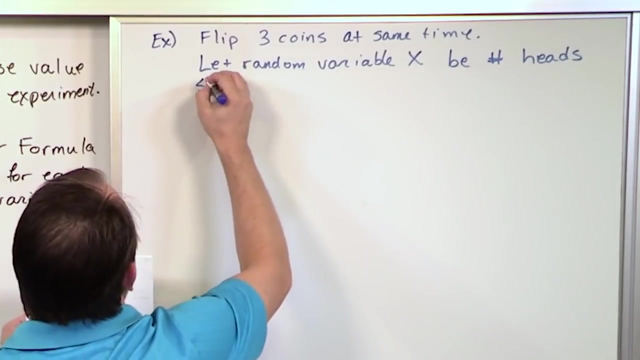 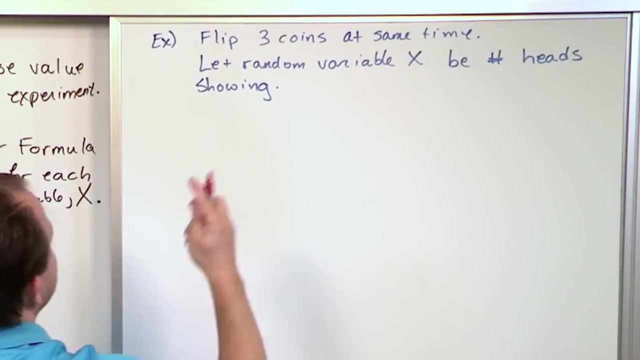 So we go flip, flip, flip and we observe the results right At same time. So then we will let random variable x be the number of heads showing. Okay, So that's our experiment. Then we're going to say: here is the discrete probability. 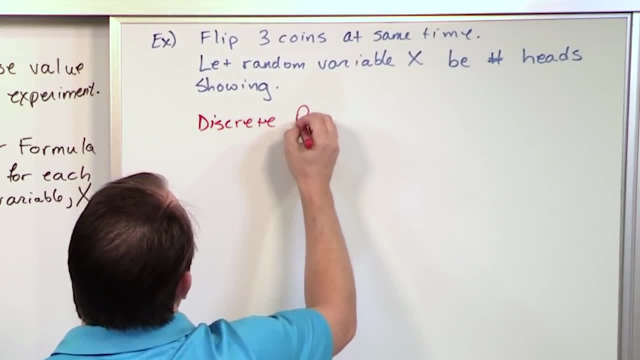 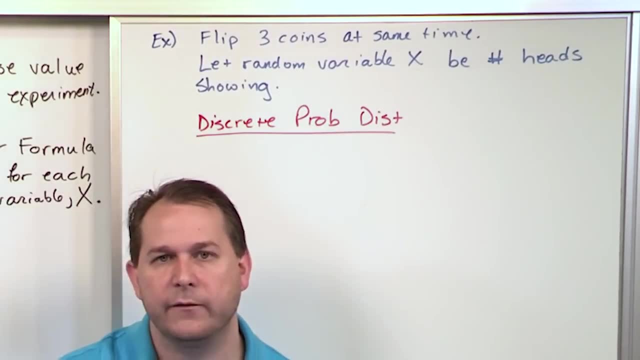 distribution. Okay, So that's our experiment. Then we're going to say: here is the discrete probability distribution. Okay, So that's our experiment. Then we're going to say: here is the discrete probability distribution of this experiment. So make sure you understand what's happening. I've got three quarters in my hand. 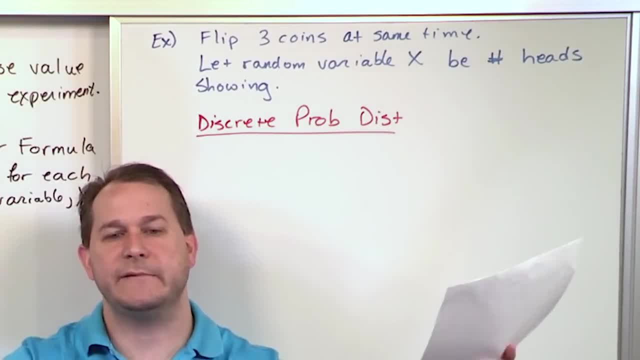 This is the easiest way to do this: Three quarters. I throw them up. They all go up at the same time. They all land on the ground. Sometimes I'm going to get all heads. Maybe I'm really lucky. I get all heads. 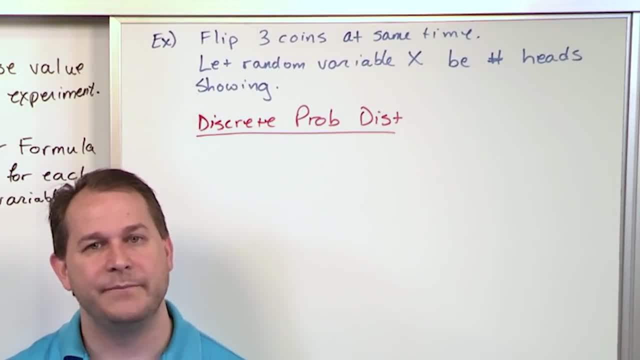 Sometimes I'm going to get all tails, But most of the time it's going to be a mixture of those two. I'm going to get some heads and some tails. Sometimes I'll get one head and two tails. Sometimes I will get one tail and two heads. 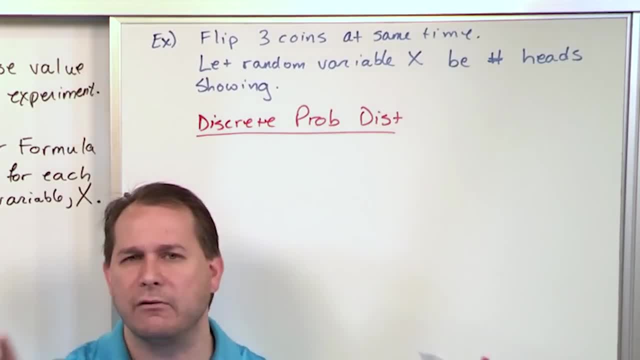 Now what we're trying to do is figure out all the different outcomes of this experiment. when I have three coins, all the different outcomes, And what is the likelihood of getting any of these different outcomes, The likelihood being the probability. That's why we kind of did a little probability refresher in the previous section. 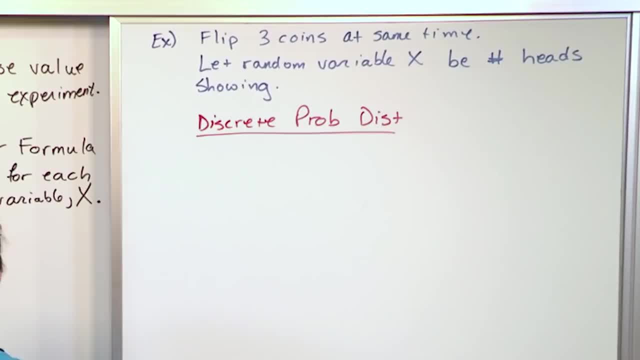 So the way to do this a lot of times, especially in the beginning, is to draw a picture. Now, you can't do this with a lot of problems, but you can do it in the beginning to solidify. So when I do this experiment- I already said that- sometimes, if I'm really lucky, 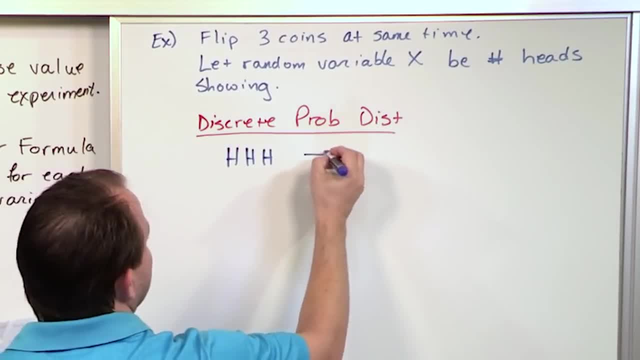 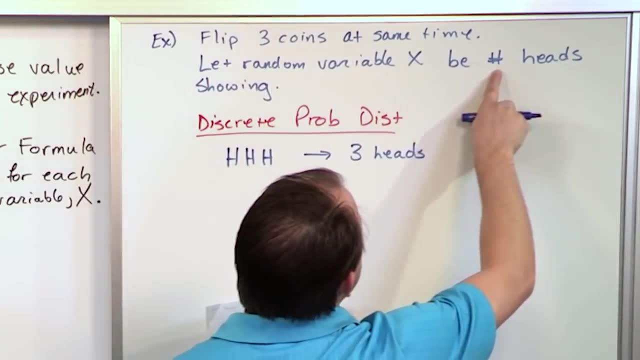 I'm going to get three heads in a row, So let me just kind of write over here: this is three heads, Because, notice, the experiment says I flip three coins at the same time. Let the random variable x be the number of heads. number of heads showing. 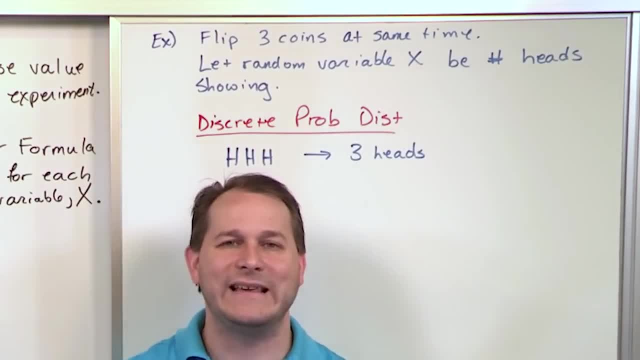 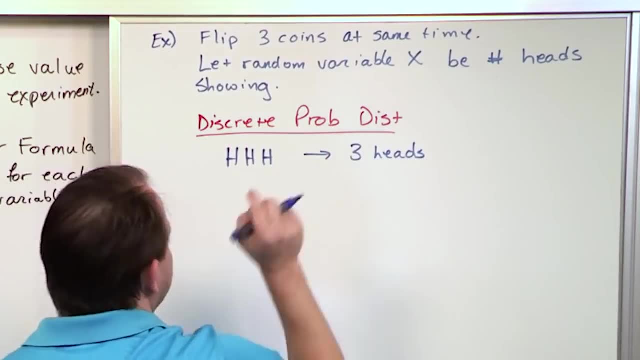 the random variable that I care, which means the outcome of the experiment that I care about, is just how many heads are showing. That's what I care about. So in this case, I write down: if this falls, I get three heads. 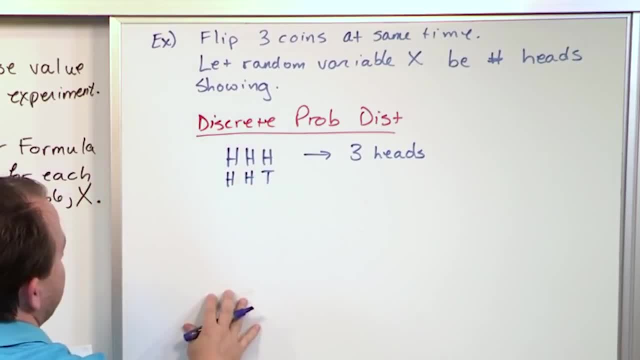 But of course I could have head, head, tail showing, in which case I only get two heads. But I could also have heads, tail heads, like this, which will also be two heads showing. But then I can also have head, tail, tail, in which I only have one head showing. 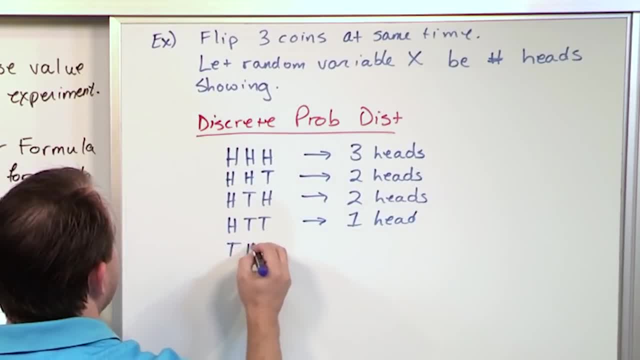 And then I can have tail, head, tail. I only get two heads showing, All right, head, head. and then I have again two heads showing. Then I can have tail, head, tail, which will only give me one head, And then I can have tail, tail, head, which is one. 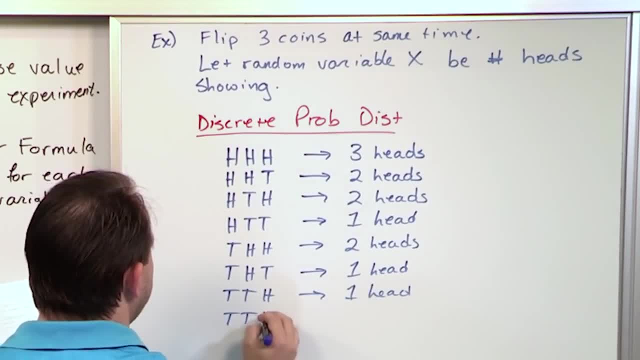 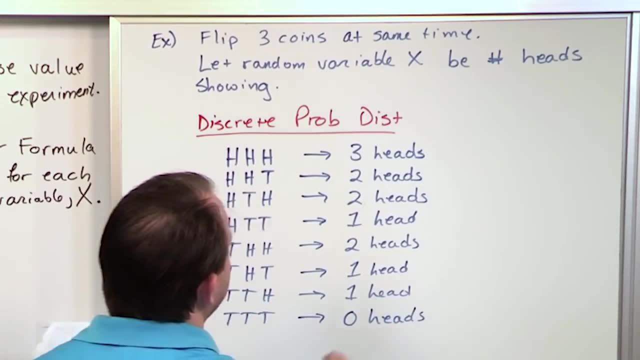 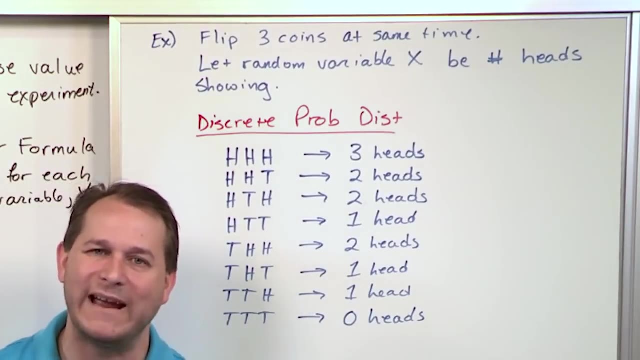 head, And then I can have tail, tail, tail, which is the other way. I'm really lucky. Let's say, three tails in a row and I get zero heads. All right, Effectively, this kind of is a raw representation of the outcome of the experiment. Now remember the random variable. 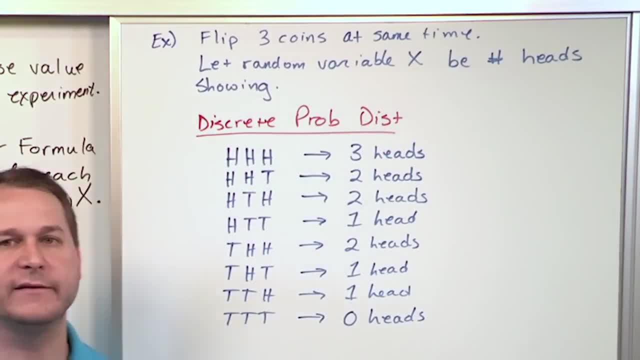 I care about is how many heads. So for every single possible outcome, I have outlined every outcome that can possibly happen. No other outcomes can happen other than what I've written on the board. There's one, two, three, four, five, six, seven, eight possible outcomes. 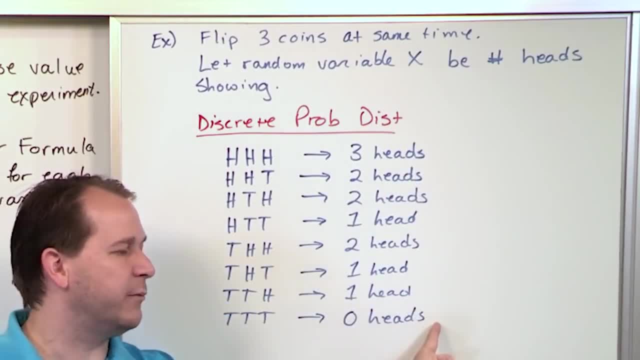 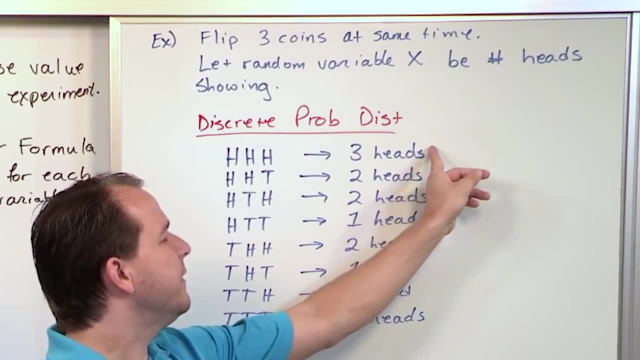 And for every possible outcome, I have figured out what my random variable value would be, which means the outcome of the experiment or whatever I care about. Now. notice that there's only one head, One way in which I can get three heads, Only one way that that can happen. There's also: 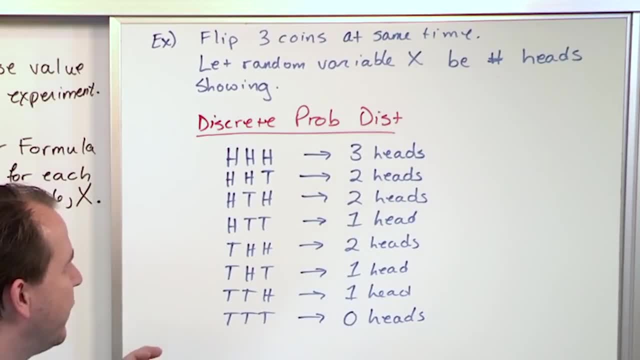 only one way that I can get three tails. So when you look at this and if you're interested in the number of heads, then you can just tell by looking at this that the odds of getting three heads is lower than everything else, Because there's only one way on the board. 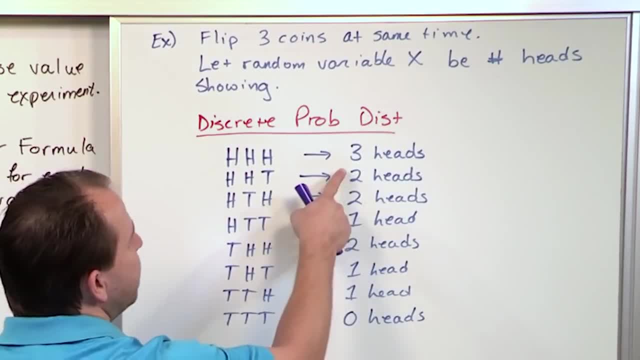 one combination that gives me three heads. But if you look at the number two, I get two heads here. two heads here, two heads here. So that's a little more likely to get two heads Also. I get one head here, one head here and one head here. That's also pretty. 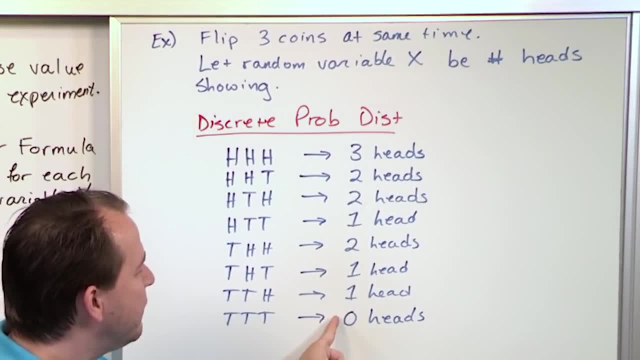 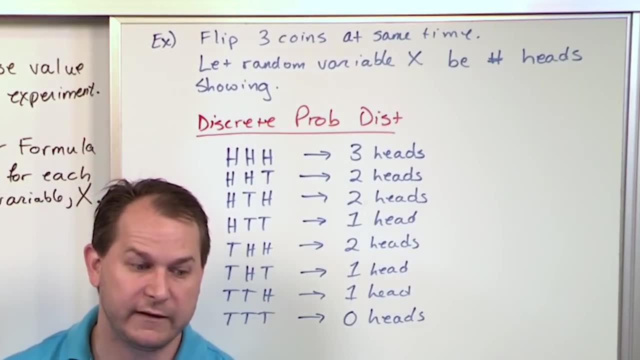 likely because there's more ways in which that can happen. And then getting zero heads is also pretty unlikely because there's only one way in which that can happen. So you can see that by flipping these three coins and if I'm interested in the number of heads, 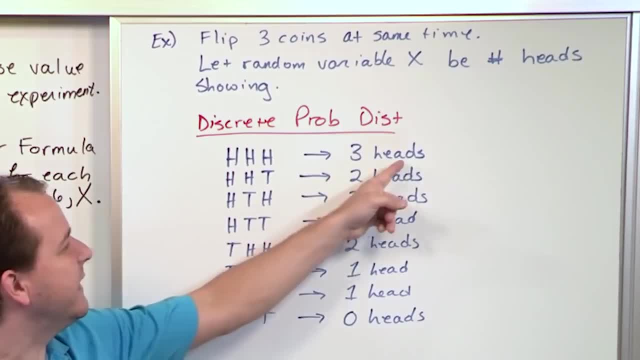 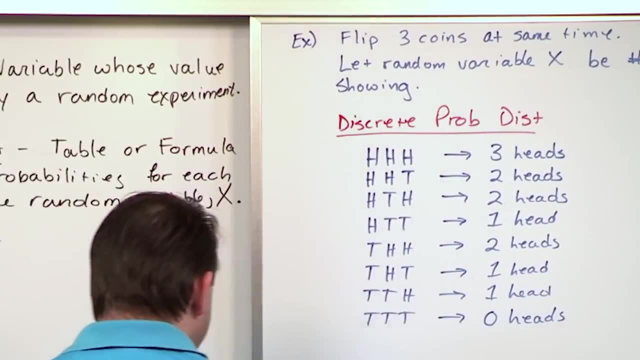 sometimes you can just tell by looking at this. it's going to be more likely to get a mixture of heads and tails where I have two of one and one of the other. So this is sort of the raw information, but when we write the probability distribution, 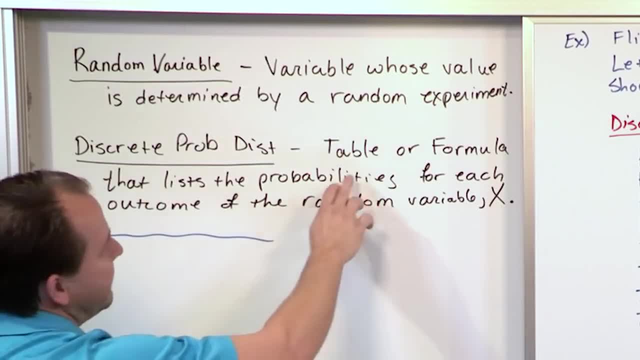 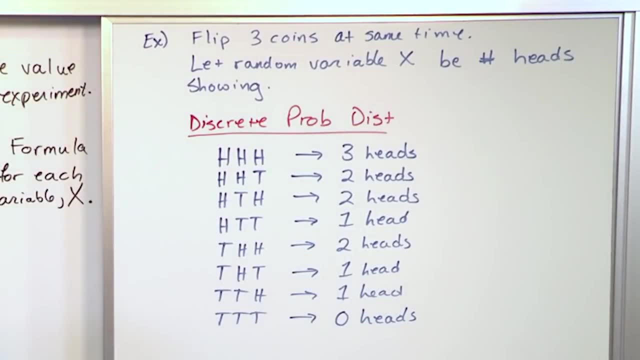 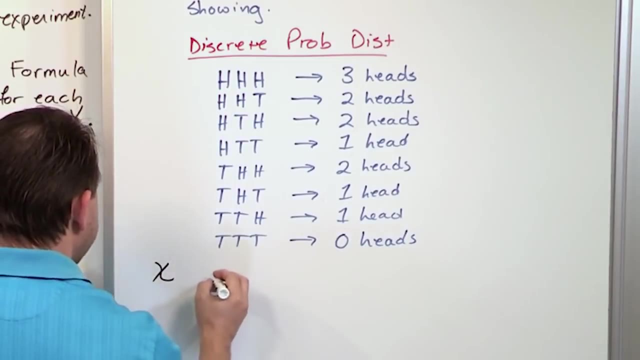 it says it's a table or a formula that lists the probabilities. I haven't listed any probability here because I just listed the raw outcome. If I want to write down the actual probability, then I might do something like this. I'll do X. X means the outcome of the experiment. 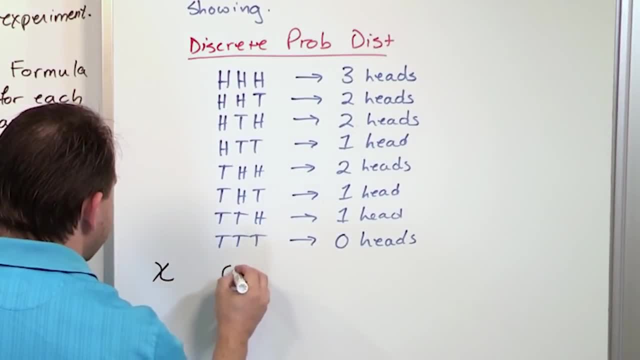 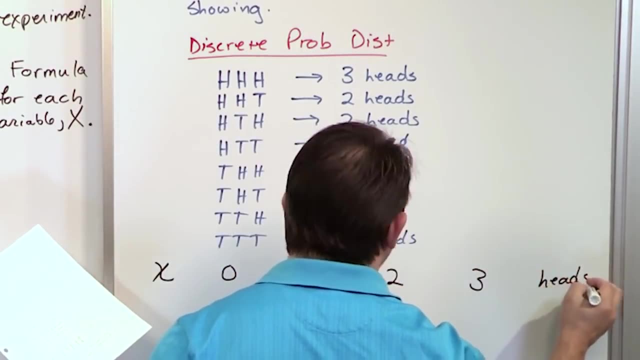 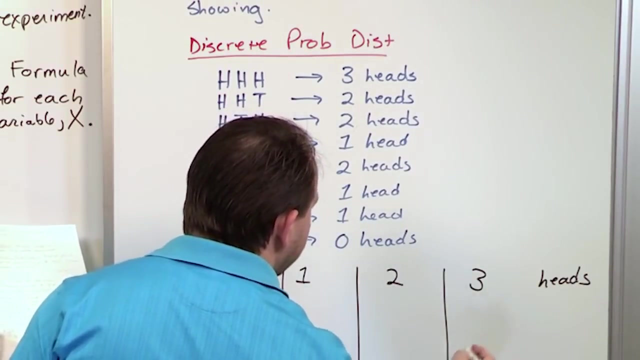 Notice this is like a cursive X. The outcome of the experiment can be zero heads, one heads, two heads or three heads, And I'll just remind you, over here I'll put heads. So I'm going to make a little table here just like this. All right, This is a little. 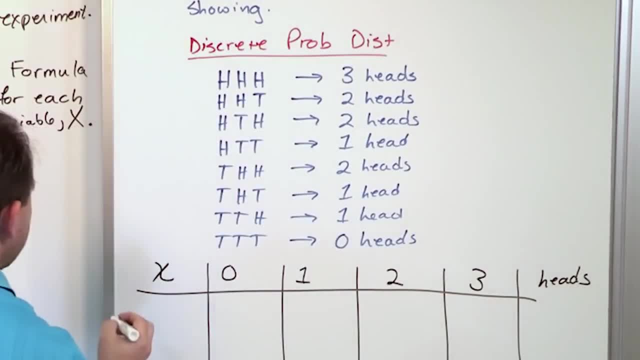 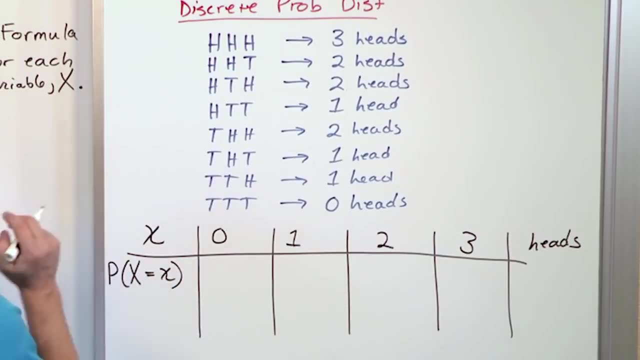 table. Now those are the possible outcomes of the experiment. So what would be the probability of my random variable capital X equaling lowercase x? This is a lot of the ways you'll see it written in a book. Basically, you're saying what's the probability that I'm going to get. 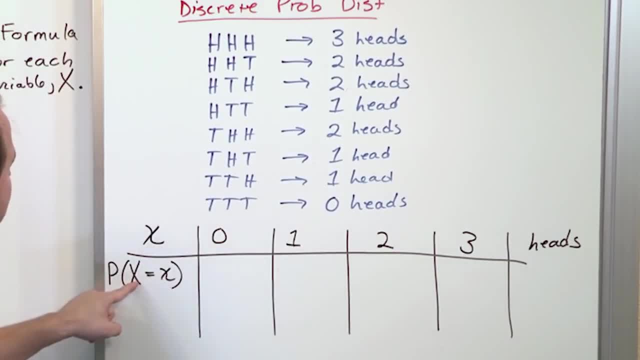 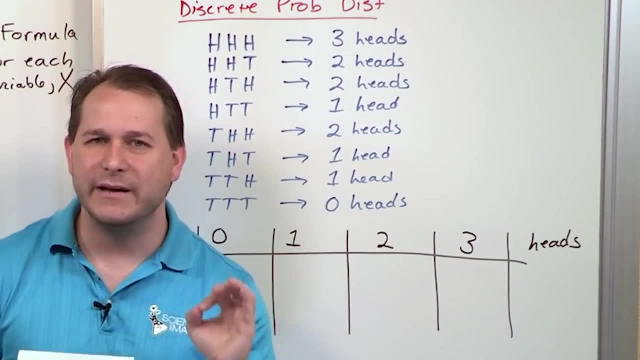 a random variable equal to zero, a random variable equal to one, random variable equal to two and a random variable equal to zero, A random variable equal to three. We've written all this stuff down on the board, but we didn't write it in terms of probability. Remember, I said, in terms of basic probability, the 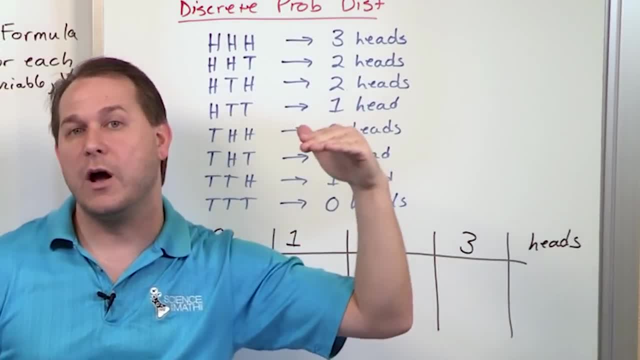 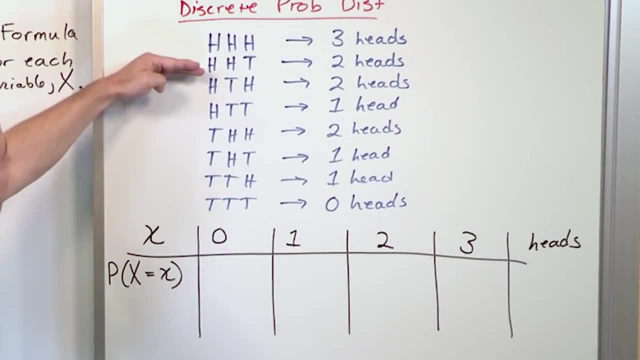 probability of an outcome is the number of ways in which I can get what I want, like when flipping a coin. there's only one head and there's two possible outcomes. Here there are eight possible outcomes. So if I want the probability of zero heads, it's only one. 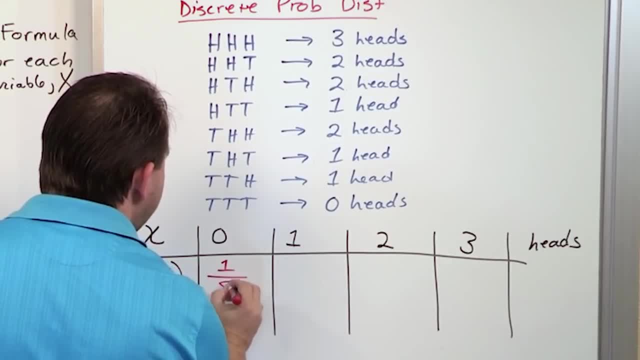 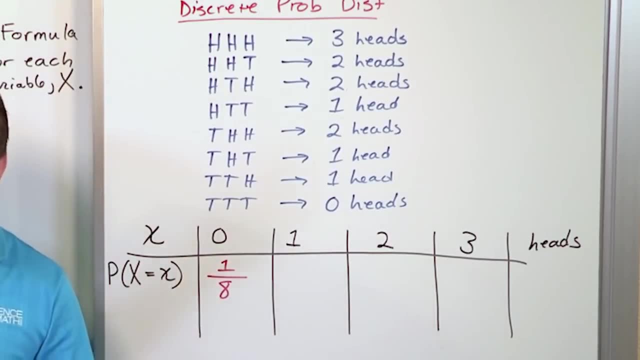 way in which that can happen. The probability of getting zero heads is one eighth, and I can convert one eighth to a decimal, just like .5 or .3 or whatever, and I will get that. What would be the probability of getting one head? Well, I get one head here, one head here and one head here, So 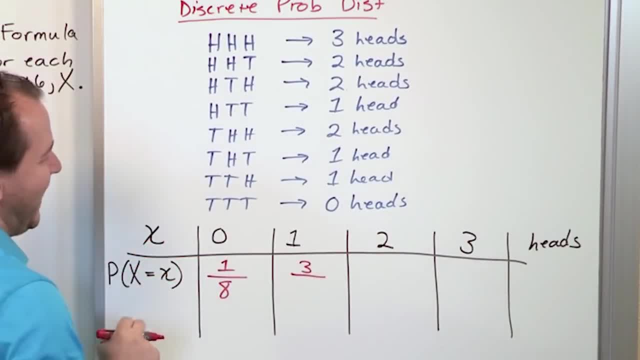 that's three ways in which I can get what I'm looking for, which is one head out of eight possible outcomes. So there's three eighths. Again, that's a number less than one, That's a decimal Right. What's the probability of getting two heads? Well, I get two heads here, two. 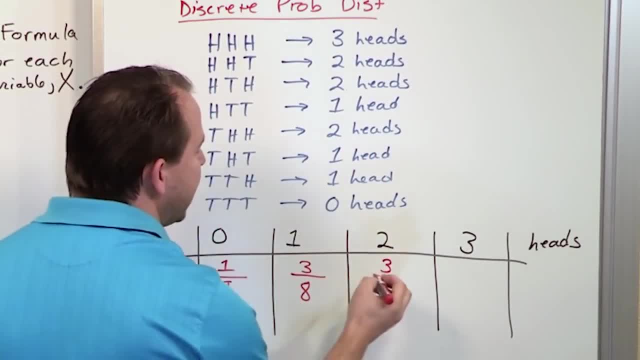 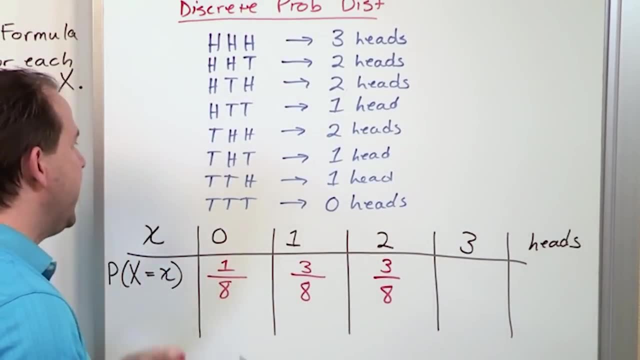 heads here and two heads here. Again, there's three possible ways to get that, and there's eight possible ways in which my experiment can end. And then, finally, what's the probability of getting three heads? I only have one way in which that can happen, and there's eight. 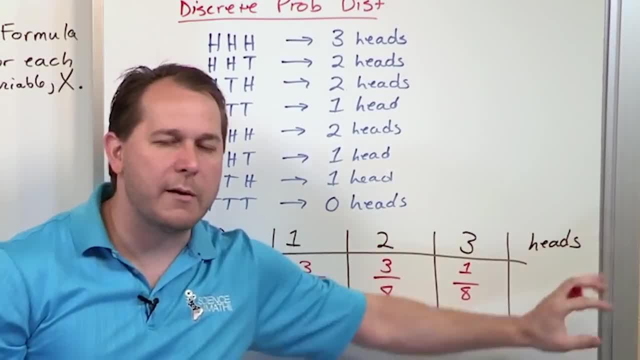 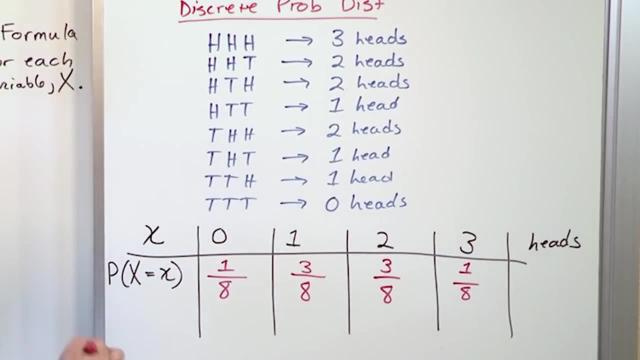 possible outcomes. This is what we call a probability distribution and, furthermore, it's called a discrete probability distribution. I'll explain what that means in a minute. but basically, on your exam or on your test or on your quiz, if the teacher gives you. 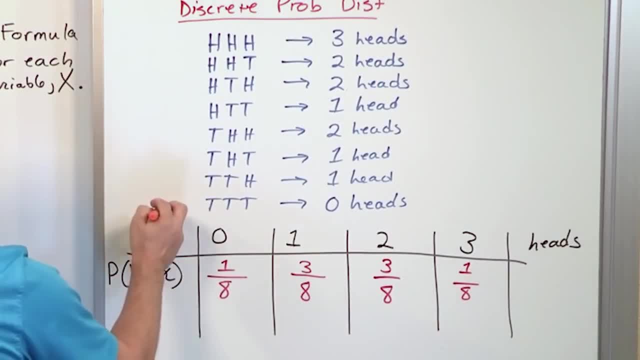 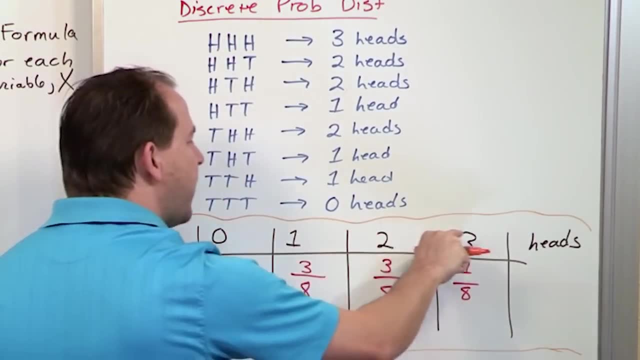 a problem like this and they say: create a probability distribution. this is what you're trying to write down, some sort of table like this where, basically, you want to list all the different outcomes and the probabilities that can be associated with those, And you 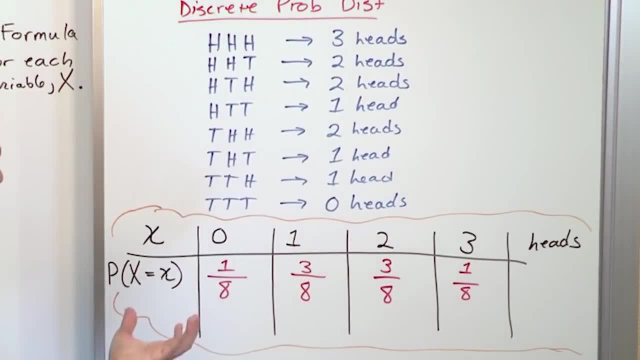 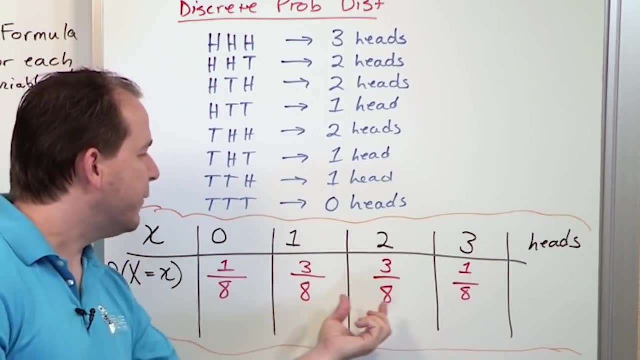 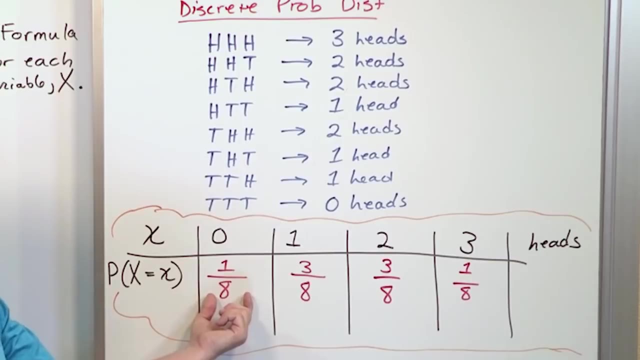 can look at this in a glance. You could sort of see it from here. but you can look at this and really powerfully see that the probability of getting one head or two heads are equal, right, Even Steven three-eighths, okay. The probability of getting zero heads or three heads is also. 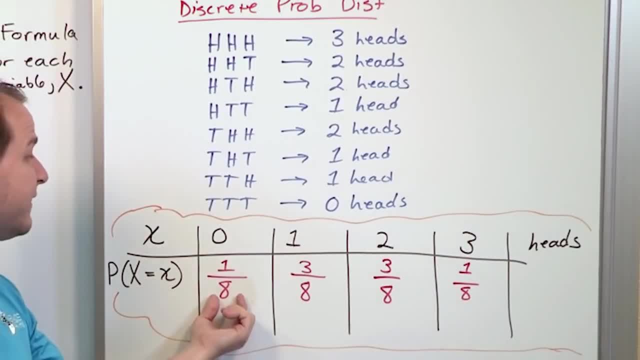 equal. That kind of makes intuitive sense as well, but it's a lower probability than this one. So I can look at this as a table and I can look at all the different possible outcomes and see that they all have different probabilities. Of course, some of them are. 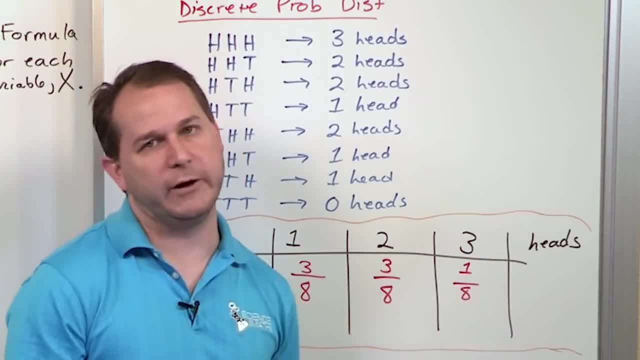 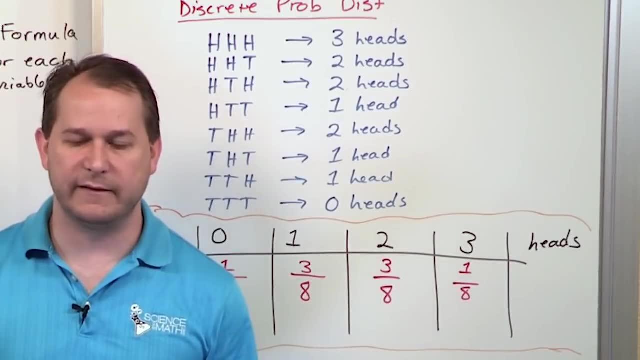 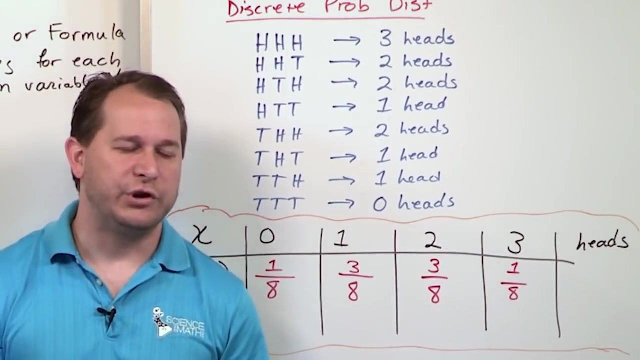 the same number, but basically there's a different probability in each column right there. So we're looking at the distribution or the spread of the probabilities Among all the possible outcomes of this experiment. Now, what makes it discrete? What does the word discrete mean? And I'm not talking about when you tiptoe in the room and you're very 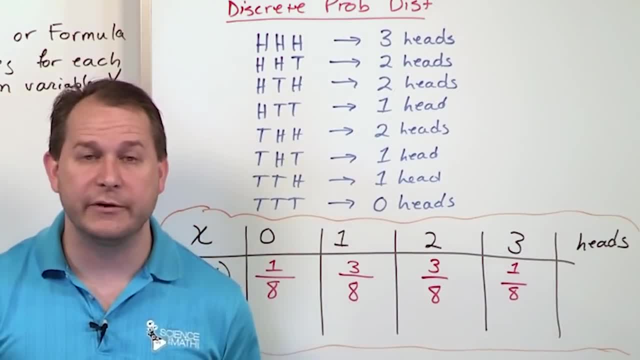 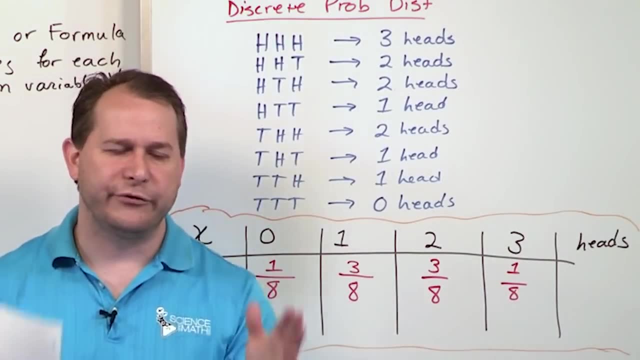 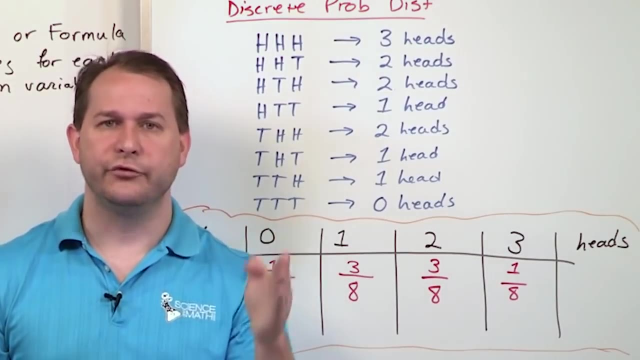 discrete about it I'm talking about in terms of math or geometry. discrete means that something is finite, Something can only take on certain values. Those are discrete values. So, for instance, when you think about integers, those are discrete numbers. One, two, three, four. 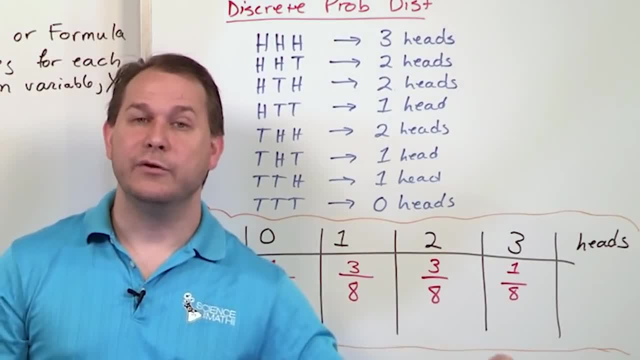 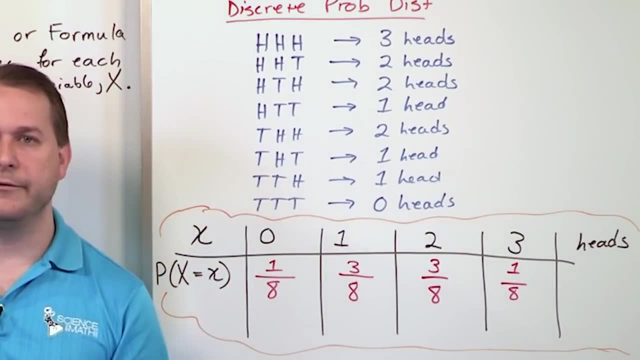 those are the integers. Zero negative, one negative two, those are also integers, They're just negative. So every whole number like that, negative plus positive, we call that an integer. Those are discrete numbers, okay, But when you start dealing with real numbers, 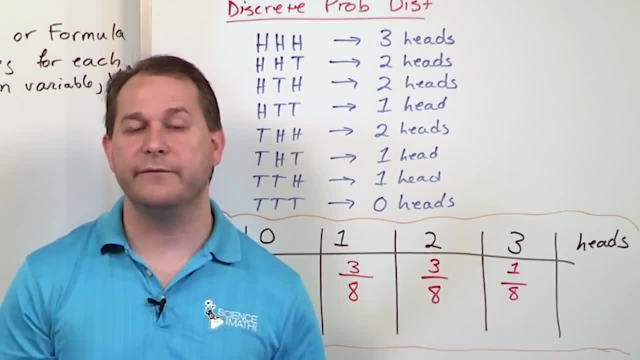 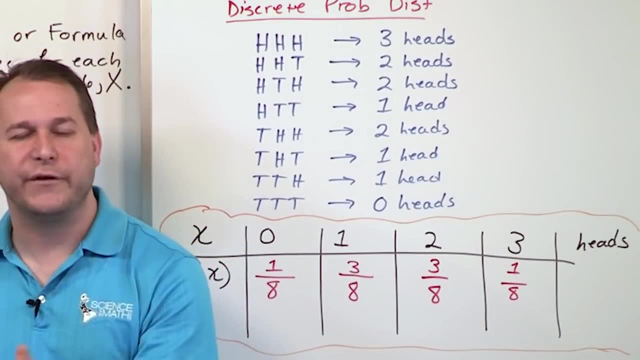 with everyday life. you can have lots of numbers in between zero and one. In fact, there's infinite numbers between, just between zero and one. There's infinite numbers Just between three and four. there's infinite numbers because you could have 3.45678910, you know whatever. 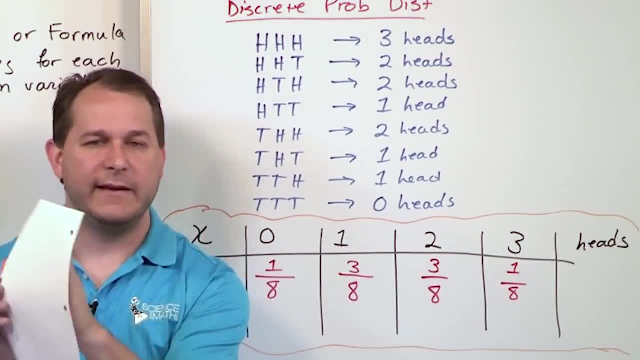 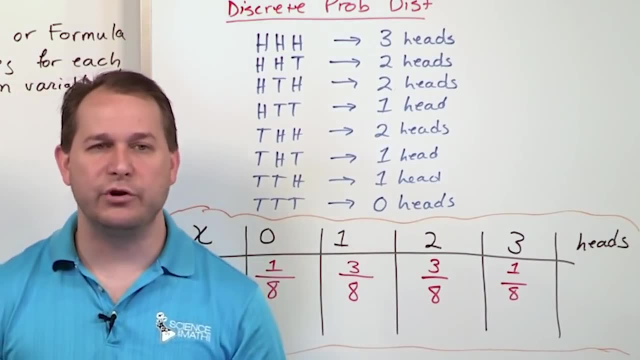 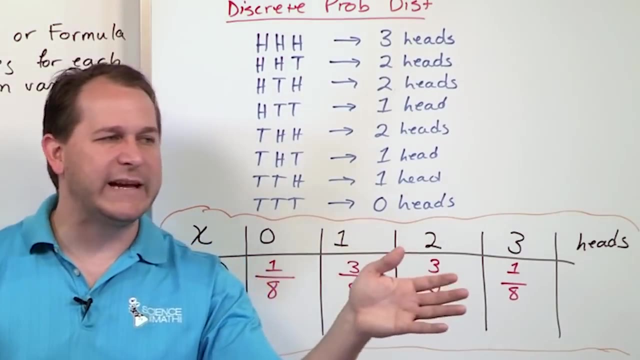 You can have infinite decimal points to split up everything between an integer pair on the number line right. So that would be called continuous. When you look at continuous values you have a problem where you can take on values that really can have any number of decimal points. 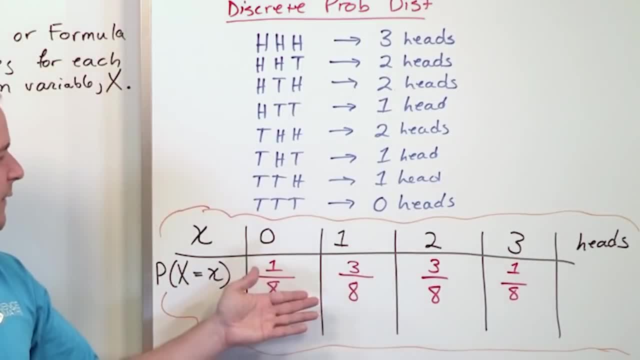 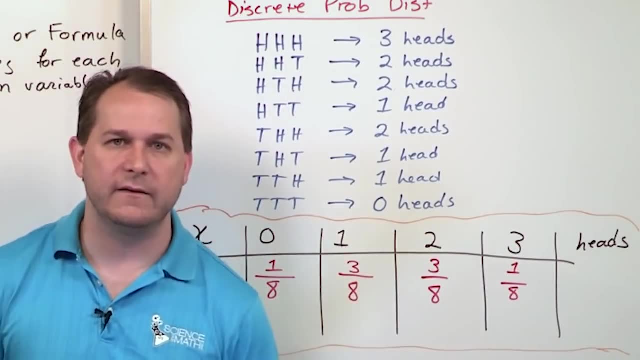 That would be continuous. But this is not continuous because the outcome of the experiment can only have certain values. You can only get zero or one or two or three heads. You can't get two and a half heads Or 3.25 heads in this experiment. You can't It just physically, you're throwing coins. 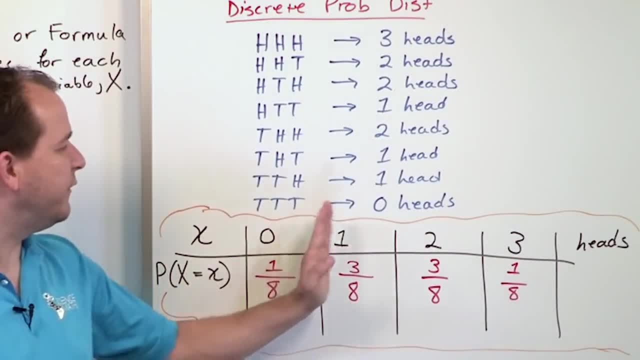 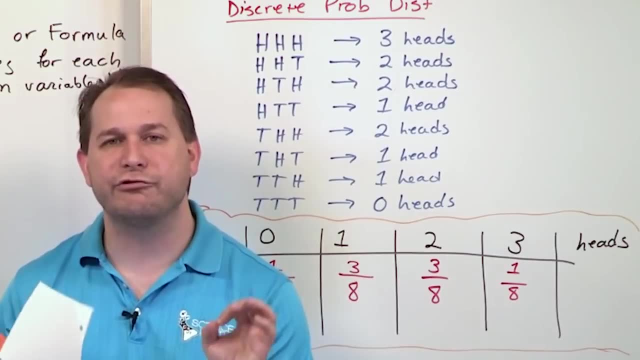 and you look at the results. So because of that, you're only going to have one, two, three, four columns, And so you can only have four probabilities. You can't have anything more or less than that. So this is called a discrete probability distribution. When 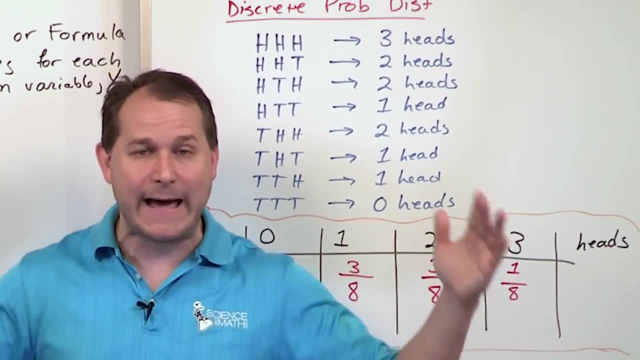 you have values where you can write it down in terms of a table and capture everything, and that's all you can get. that's called discrete. Let me jump ahead just a little bit and tell you that most of the time it's going to be the same thing You're going to 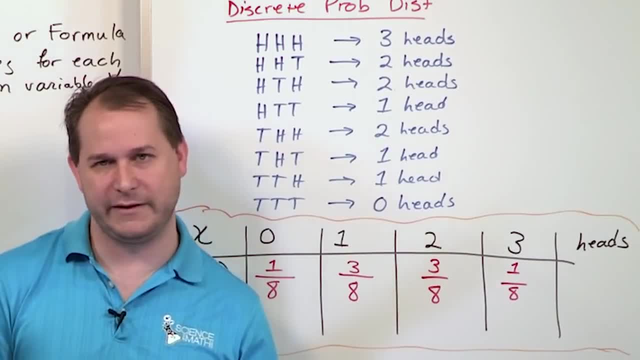 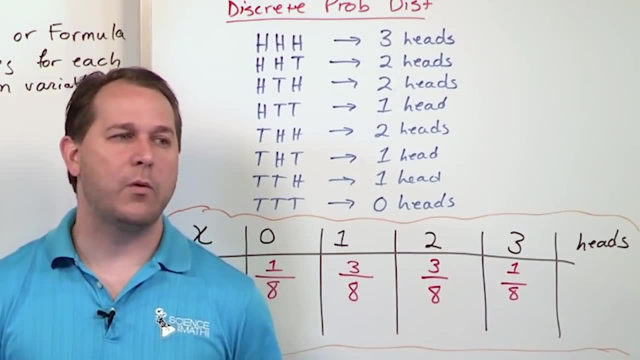 tell you that most of the time in statistics we're not going to be dealing with discrete probability distributions. We're doing this to mostly show you the idea behind what a distribution is. But in real life, what if I wanted to look at the probability of someone? 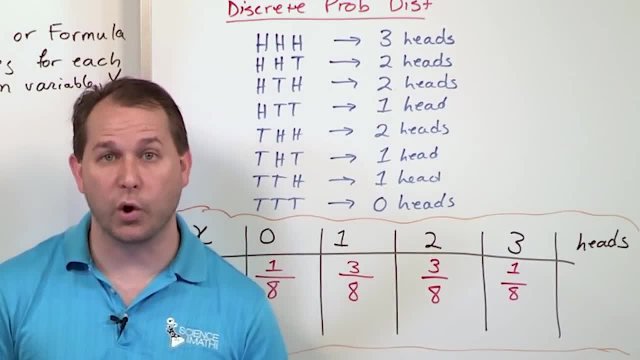 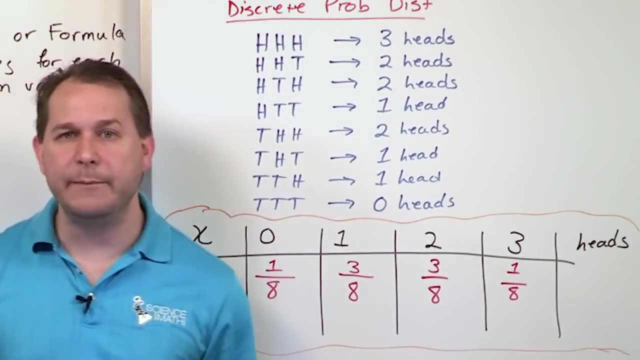 having a certain height? Or what if I took a survey and looked at everybody in the world and looked at their height And I tried to figure out what would be the probability distribution of getting different heights of people. Well, some people are going to be four feet tall. 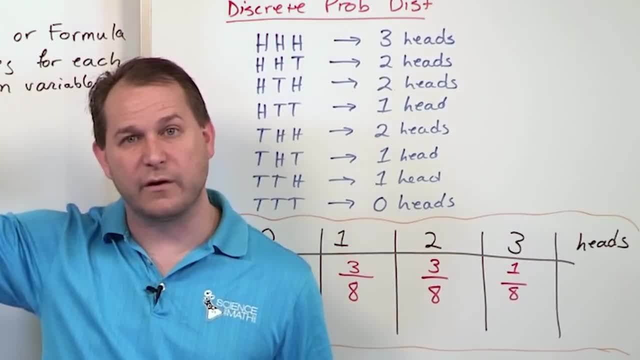 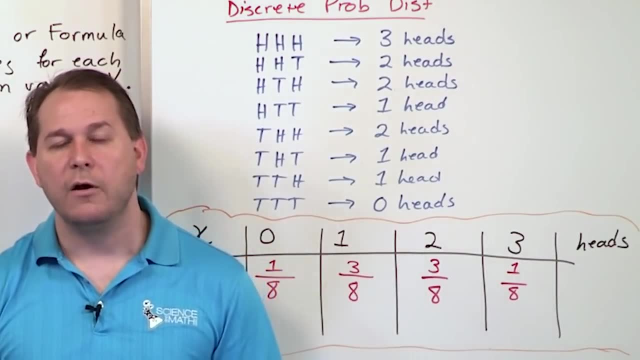 It's real small. Some people are going to be seven feet tall. That's real tall, And some people may even be taller or shorter than that. Some people may be in the middle, more like five or six feet tall, But there's always going to be people that are not exactly six feet tall. 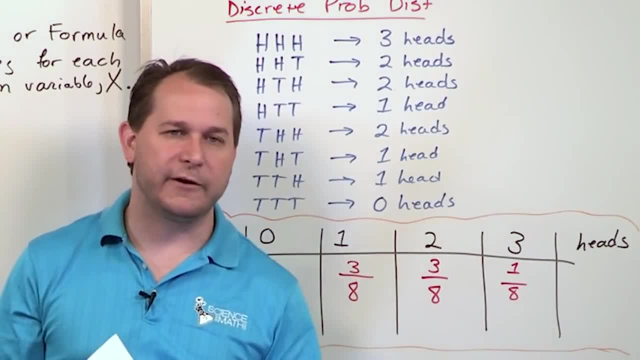 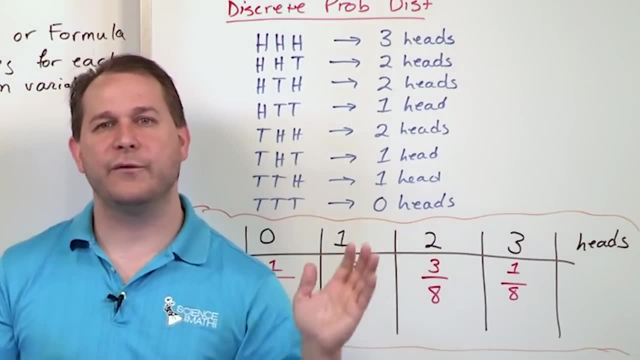 They may be 6.125 feet tall, There's always going to be people that are 5.795 feet tall. In other words, if you look at somebody and try to figure out the distribution of world heights, there's going to be basically almost infinite values in between, because height 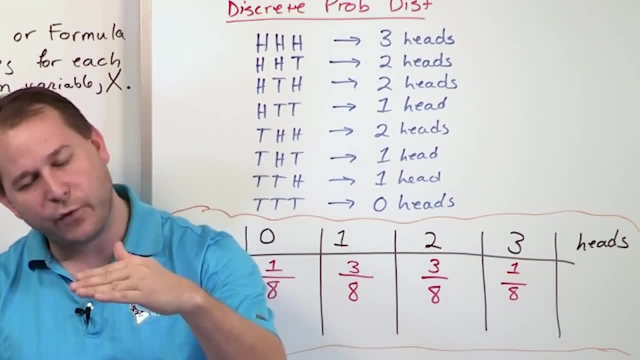 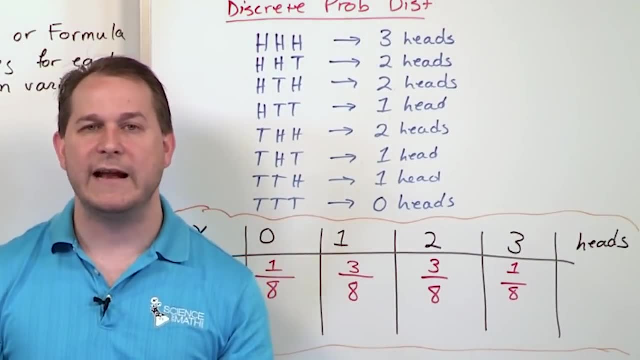 is something that's not discrete. Height is continuous. You might have somebody that's four feet, five feet, 4.5 feet, 4.75 feet, 4.8 feet. There's many, many different values that height can take. So when you look at the real world and you're trying to take surveys, 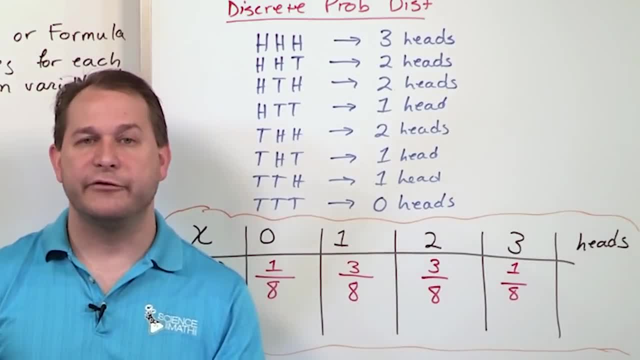 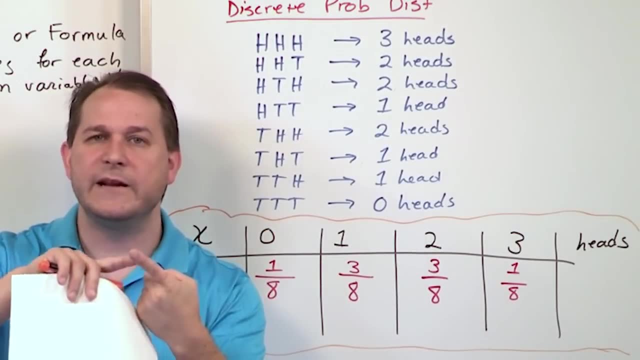 of people's height and do problems with the probability of certain height distributions in the country or the length of people's finger. there's going to be an infinite number of answers there, And so it's not discrete whenever you're talking about real-world probability. 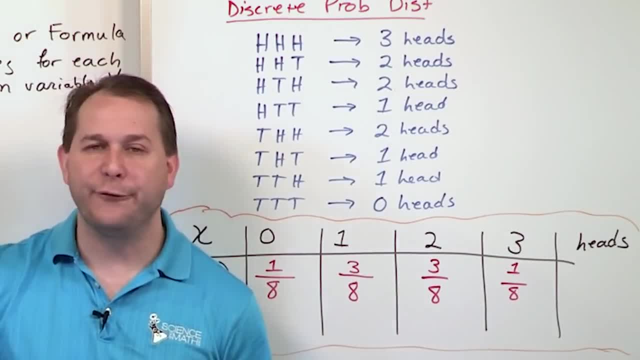 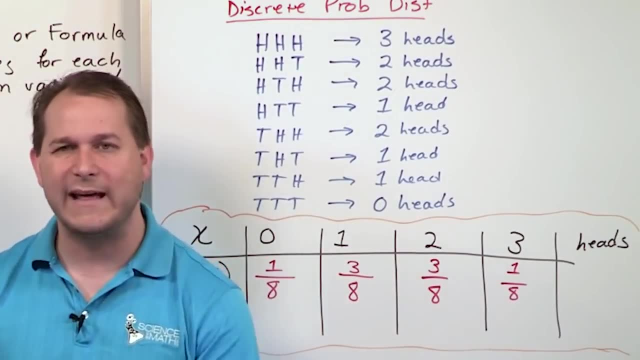 Yeah, There are problems a lot of times. That's the bottom line. So as we go forward, we're going to be continuing to talk about the probability distribution concept, But they won't be discrete. They'll be what we call continuous, And we'll get to that a little bit later, But for now, 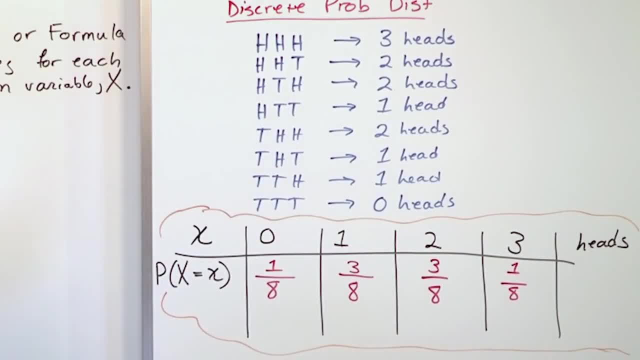 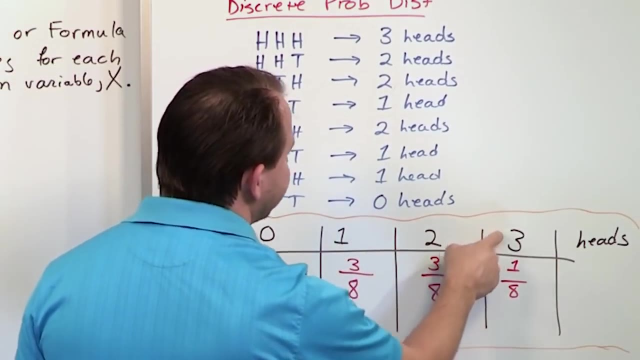 just remember, this is a discrete probability distribution. There's one thing I want to point out to you that's extremely important. Okay, Here we said: the probability of our random variable having zero heads is one-eighth. Probability of getting one head is three-eighths. Probability of two heads is three-eighths Probability. 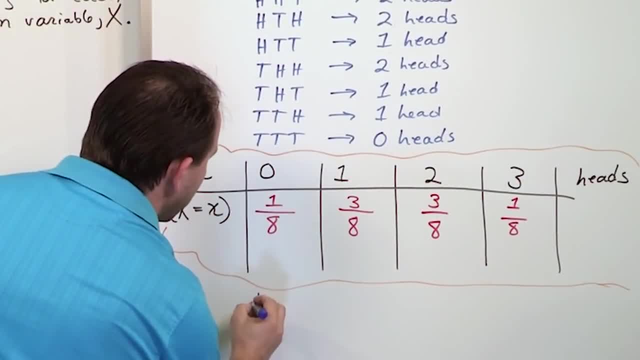 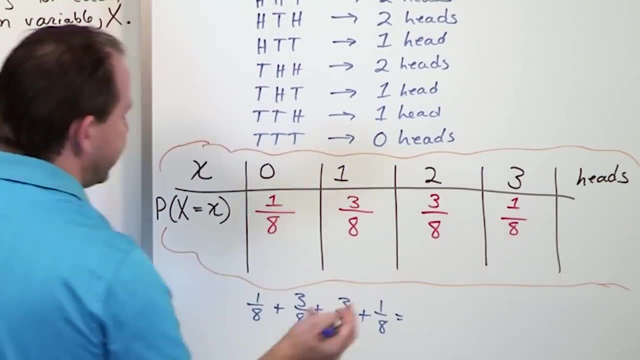 of three heads is again one-eighth. Let me show you something. What is one-eighth plus three-eighths, plus three-eighths plus one-eighth? Well, you have to bust out your fraction math. Notice that all of the denominators are eight. So that's convenient. So all we 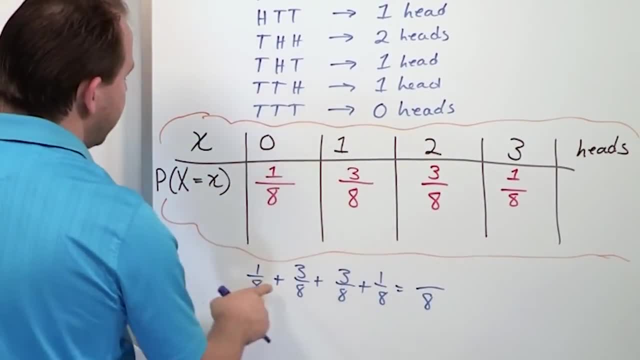 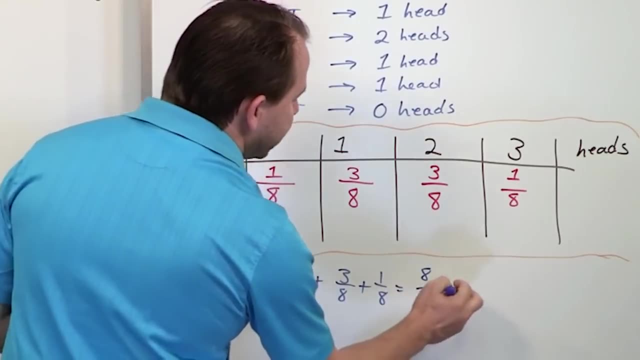 do is we put an eight on the bottom, We add fractions if the denominator is the same. One plus three is four. Four plus three is seven. Seven plus one is eight. So we get eight over eight And that equals one. When we do fractions, eight divided by eight gives: 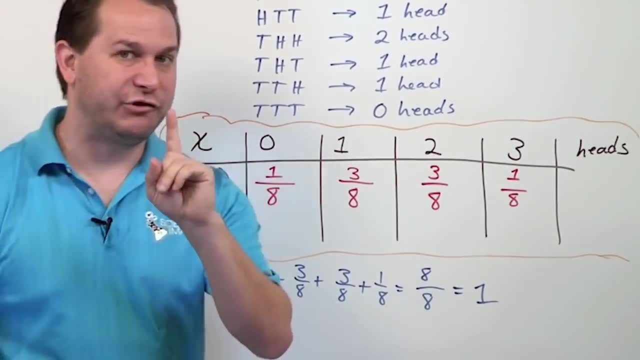 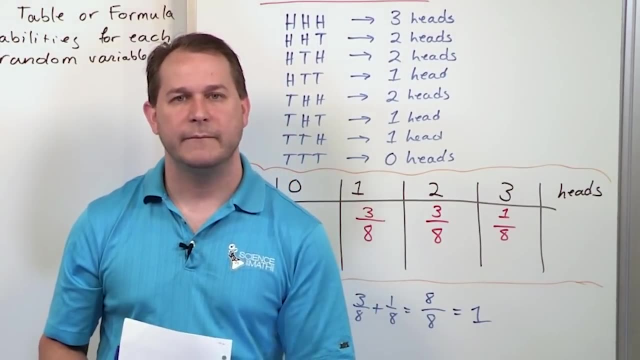 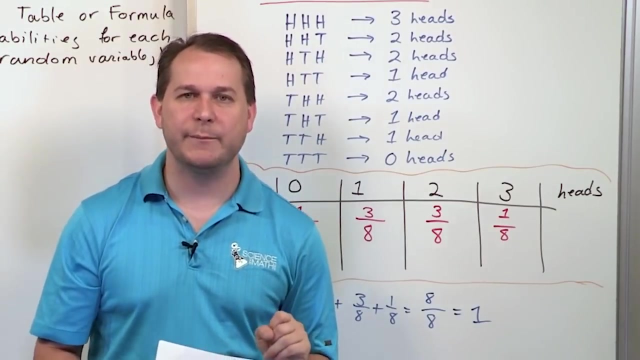 you one. So what I'm trying to say is the sum. this is extremely important. actually, the sum of all of the probabilities in our distribution equal one. Let me say that again: The sum of all of our probabilities in our distribution equal one. That's very, very important, That. 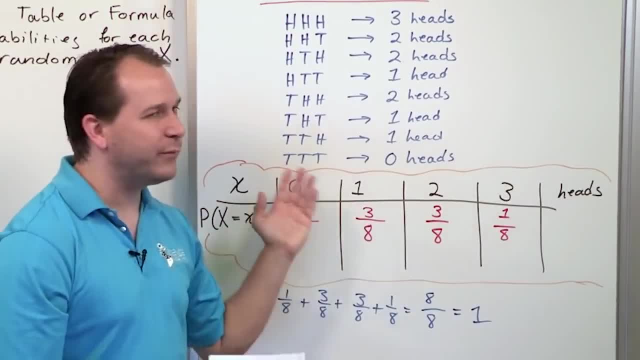 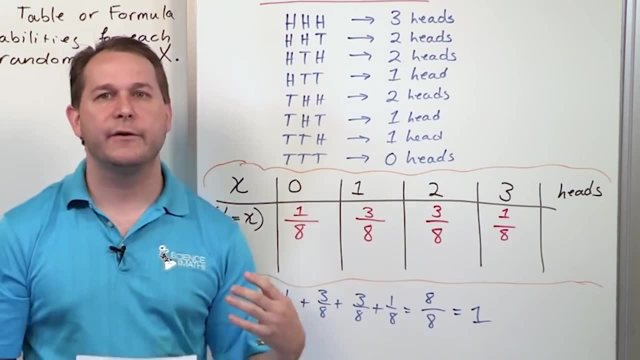 means that if I do this experiment, I'm always going to get one of these results. That's what it basically means. If I'm looking at the probability of this or this happening, or this happening or this happening, I add them all together, I'm guaranteed to cover. 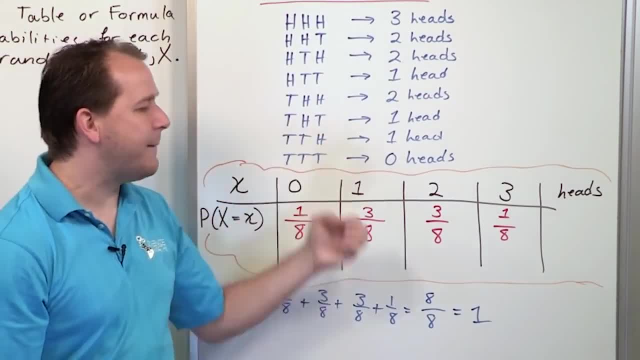 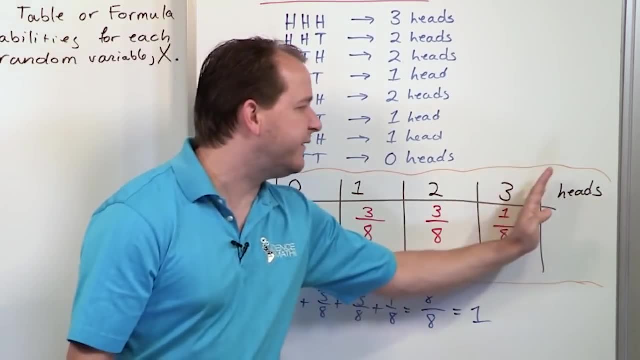 every possible answer. I'm guaranteed to cover every possible outcome because these are all the outcomes that will happen. So when I throw three coins and I get a result, I'm guaranteed to get one of these because the sum of all of the probabilities, of all the outcomes is one, which means 100%. 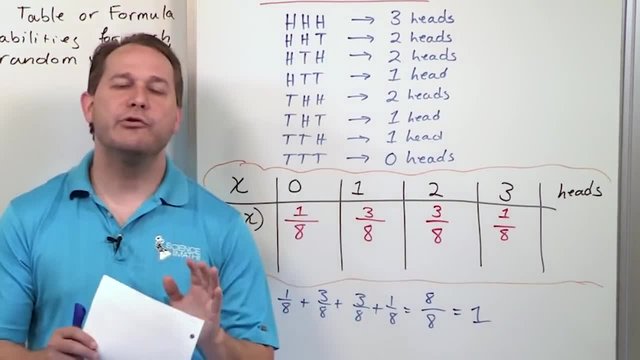 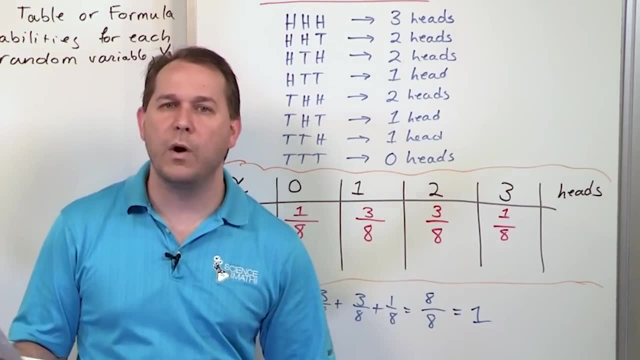 chance of happening, like 100% chance of rain. So that's going to be true of all distributions, all probability distributions. I should be able to look at the probabilities and sum them all up, and they should always equal one, because I'm trying to cover all possible outcomes. 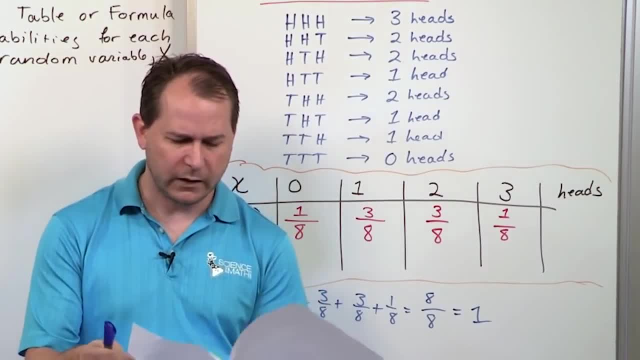 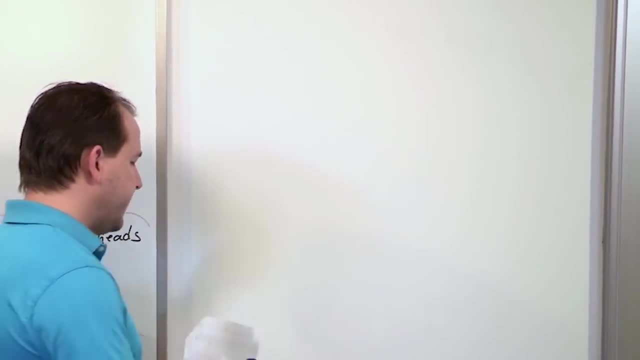 of the experiment to guarantee that it will happen. All right, let's do another one real quick. We're not going to beat it into quite as much detail, but I think it's a very good problem, so I want to do it for you. So what would 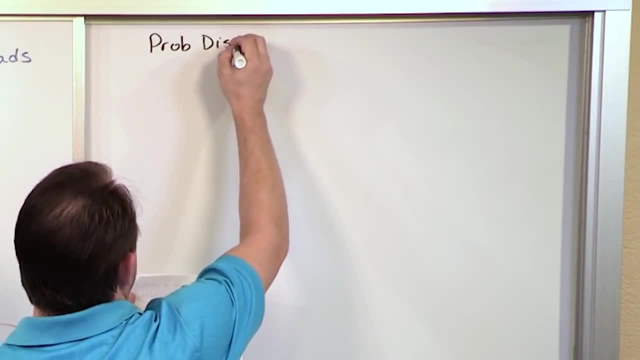 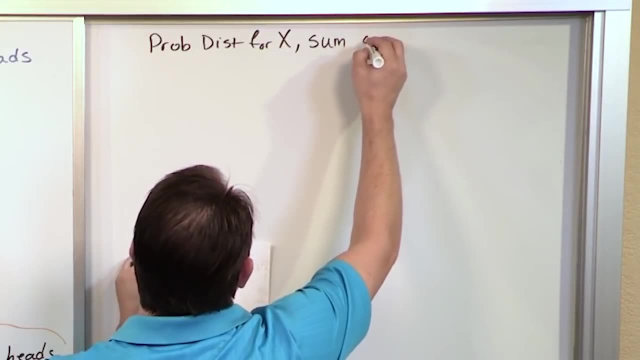 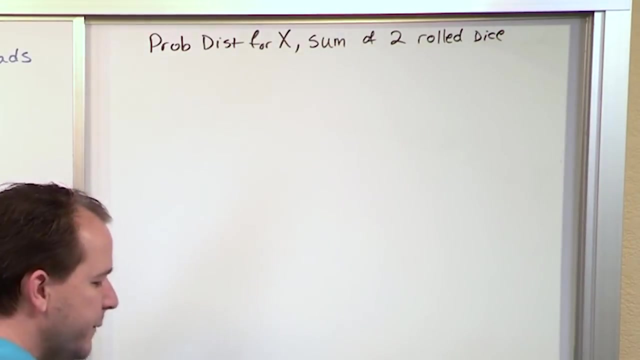 be the probability distribution for the random variable X, that's capital X, notice, which would be the sum of two rolled dice, right, Two rolled dice. And so when I'm talking about dice I'm saying one die has six faces. So we can get one, two, three, four, five, six. 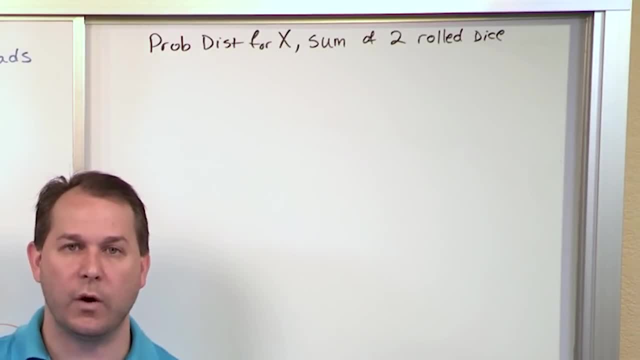 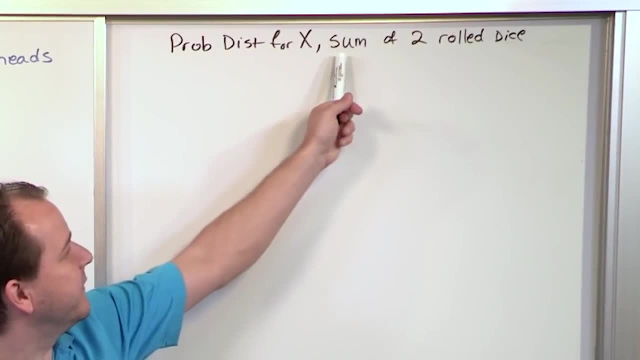 off of one die And then I roll a second die. I can get one, two, three, four, five or six off of the second die. So when I roll a pair like that and I add the two together, so I'm saying the sum of the two rolled dice, sometimes I roll two ones and I'll get an. 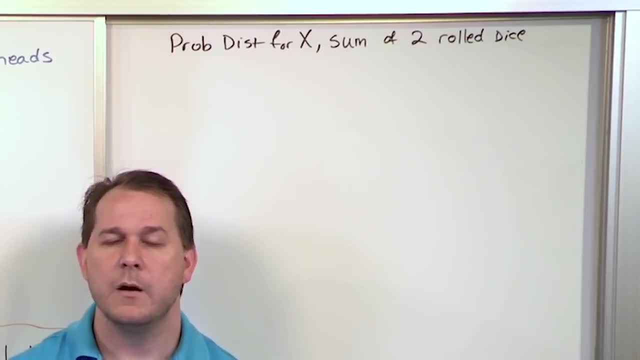 answer of two. Sometimes I roll two sixes and I get an answer of 12.. But much more commonly I'll get other combinations and I'll get the sum. I'm trying to figure out what's the probability distribution of getting different sums whenever I roll dice. So if I wanted 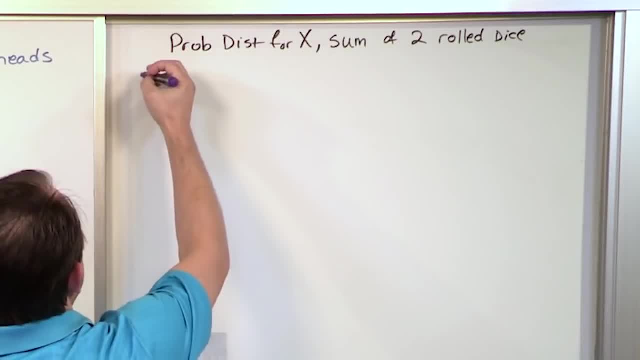 to do that, I would create a probability distribution. I'll try to squeeze it in here. it's a lot of answers, But basically I would say the probability of my random variable capital X being equal to all the possible values that I have here. What are the possible values? 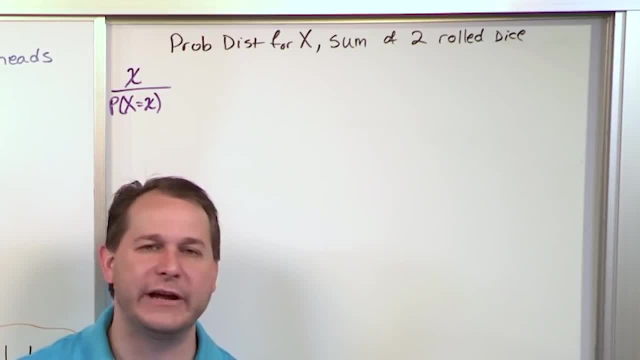 that I can take. Well, if I roll a pair of dice, I can never get a one as a sum, because I'm always going to have two die and I'm always going to have at least one on each. So you can never get a sum of one. but you can get a sum of two, right? So I can get. 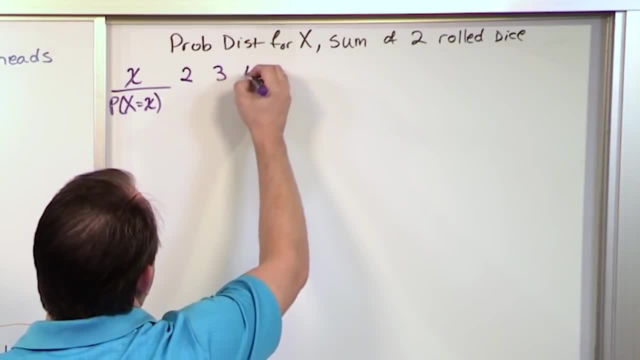 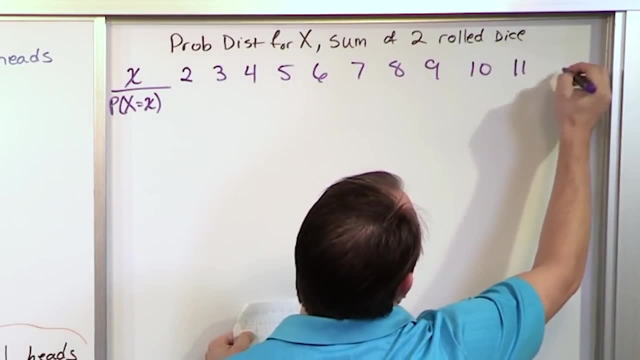 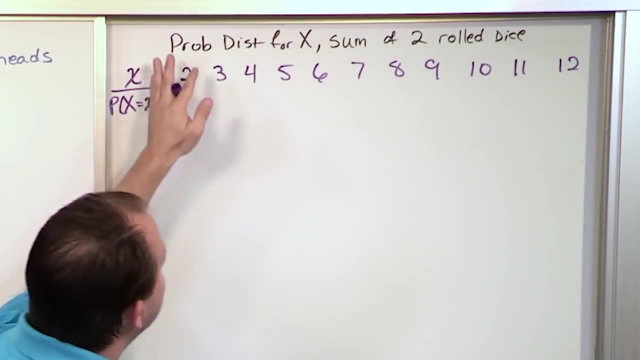 a sum of two. I can also get a sum of three. I can get a sum of four, five, six, seven, eight, nine, ten, eleven and twelve. The maximum sum I can get is twelve if I roll six and six. So the sum of all of the different ways in which I can get you know if I roll. 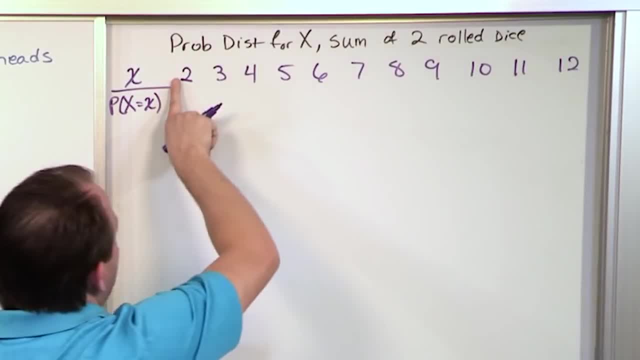 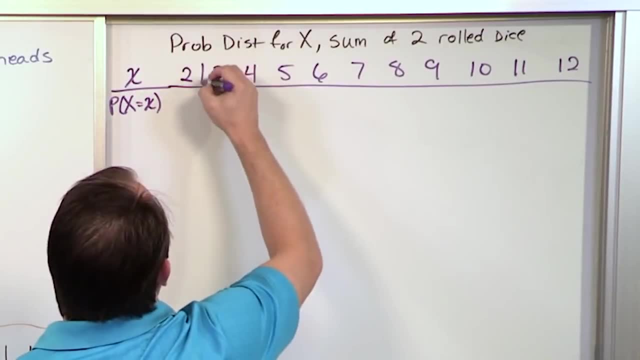 two dice is really going to be one of these answers. I can never get a one and I can never get a thirteen or higher, So let me draw this like this and let me make this into like a little table, because remember our discrete. 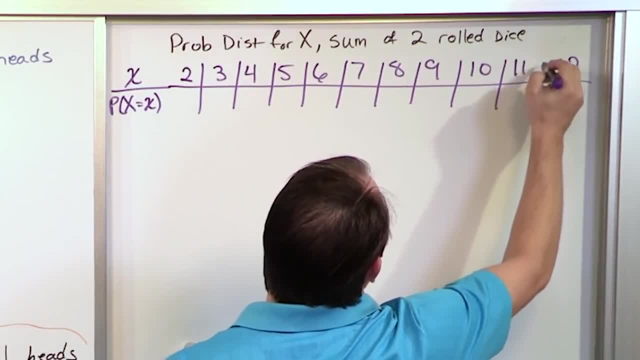 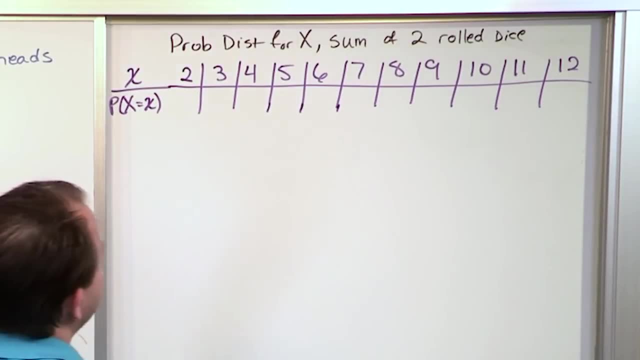 probability distribution should look like a table almost all of the time. All right, So let's go and look at this here. Let's just take a couple. We're not going to work out the answer for every one, but let's look at a couple. Let's look at the number two. How? 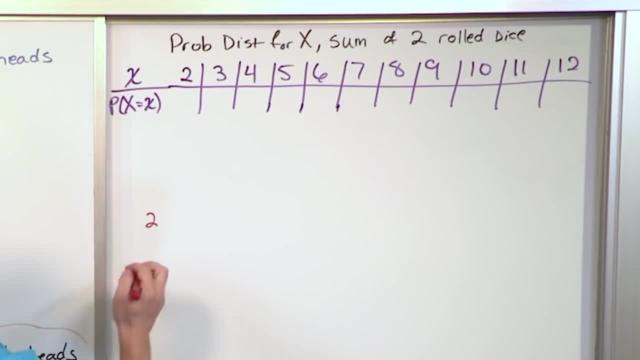 can I get the number two Right? So the only way in which I can get a number two is to get a one on one dice plus a one on another dice. Right, I can get a one plus one If this ended up being one plus two. 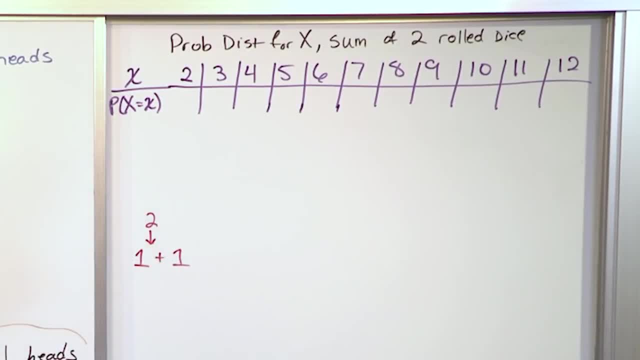 then it wouldn't add right. So the only way in which you can get two is one and one. So, as far as combinations go, there's only one way in which I can get this guy to add up, and there's thirty-six different combinations of the ways in which the dice can roll. The 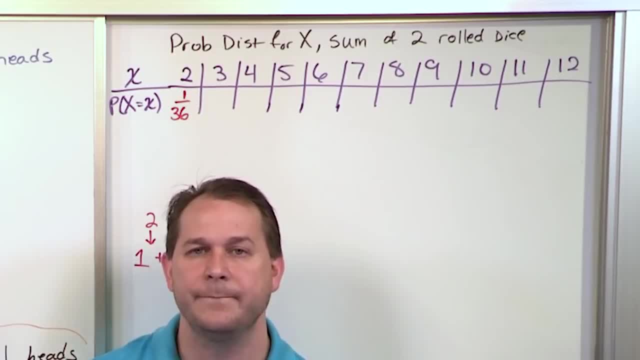 reason there's thirty-six of them is because there's six faces on one die And six faces on another die. Six times six means there's thirty-six ways in which the two dies can land. All right, Thirty-six different possible outcomes in which they can land. 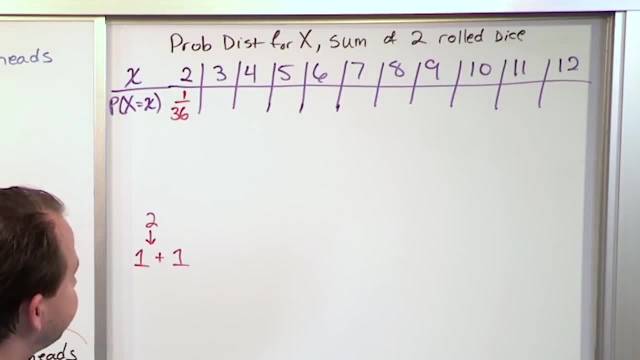 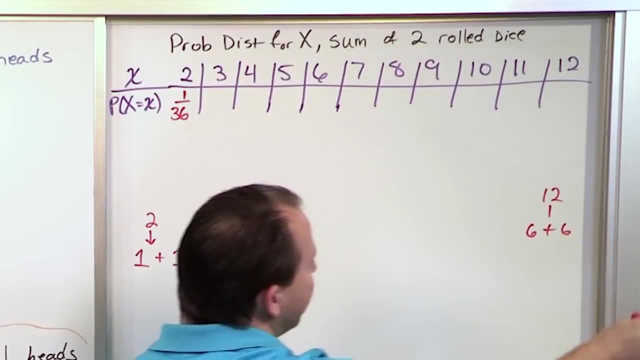 Only one of those outcomes will yield a sum of two. Okay, Similarly, look way over here When you look at the number twelve. the only way I can get that is six plus six. There's no other way I can add to twelve because the 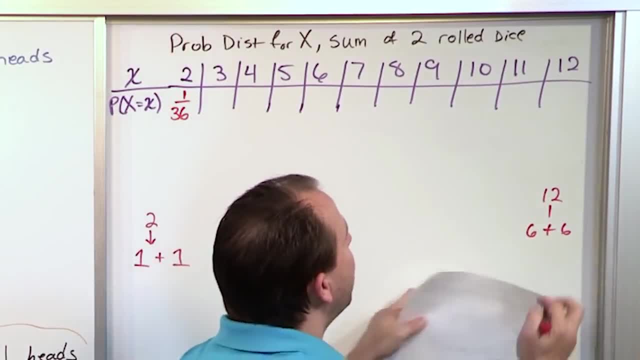 dies only go up to six, All right. So there's only one possible outcome here: to give me a twelve. But there's thirty-six plus six, All right. So there's only one possible outcome here: to give me a twelve, but there's thirty-six. 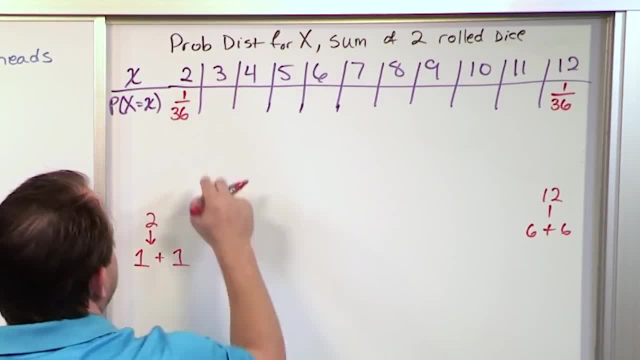 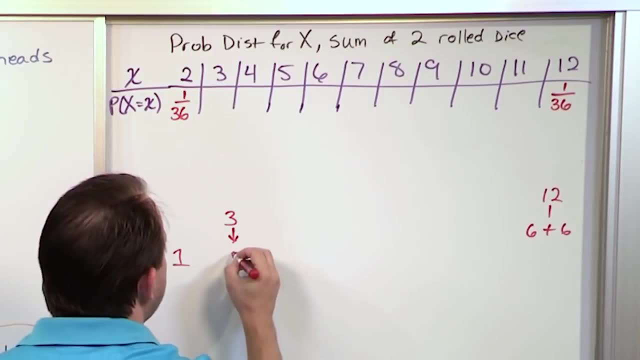 possible ways in which the die can be rolled, And then we'll just do this one as sort of a last one. If you look at the number three, how can I get the number three? How can I get the number three? Well, one die, I can get one plus two, okay, And the other die. 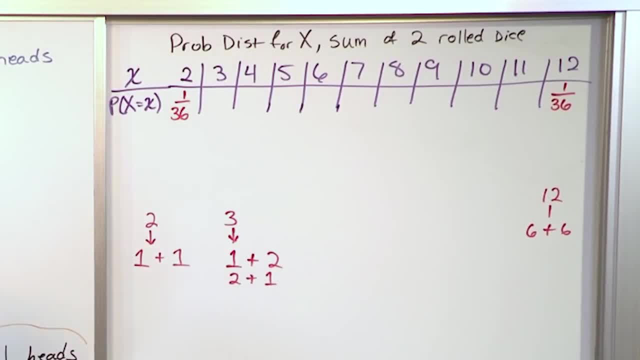 I can get two plus one. Those are the only ways in which I can roll this pair of dies to get the sum of three. It's the only ways in which it can happen. I can get a one on dice A and a two on dice B, or a two on dice A and a one on dice B, So there's only two. 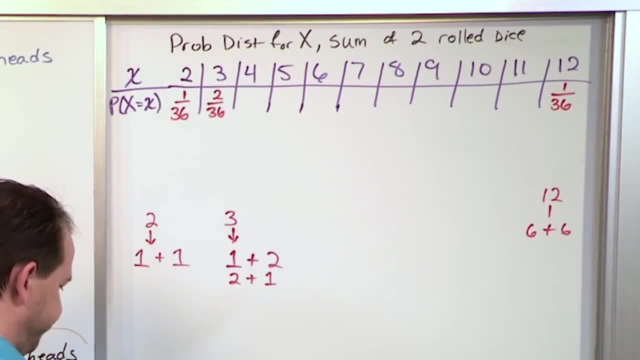 possible ways. I can sum to three, again out of 36.. Again out of 36.. So you can see what you end up having to do through here. I would have to go look at the number four and I'd have to go figure out: okay, how can I get the number four to be summed together And 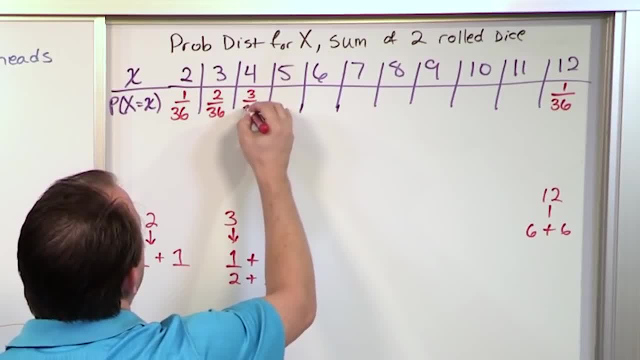 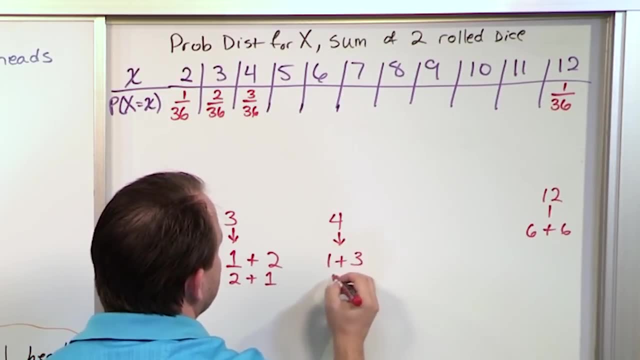 you'll find that there's only three ways in which to sum to number four 36.. In fact, I can just show you real quick How can we get to the number four. Well, we can do one plus three, We can do three plus one, We could do two plus two. Those are the only. 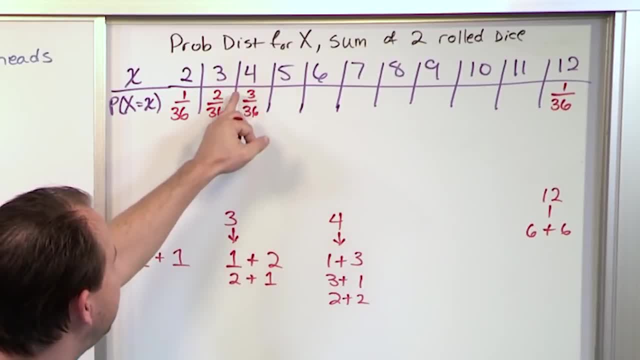 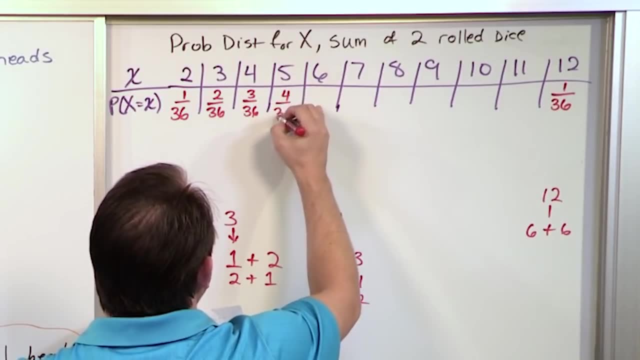 ways in which I can add to the number four. So there's three outcomes that yield a sum of four. There's 36 possible outcomes, So I'll just fill in the rest of the chart For the number five. there's four ways in which that can happen. out of 36 outcomes, This one 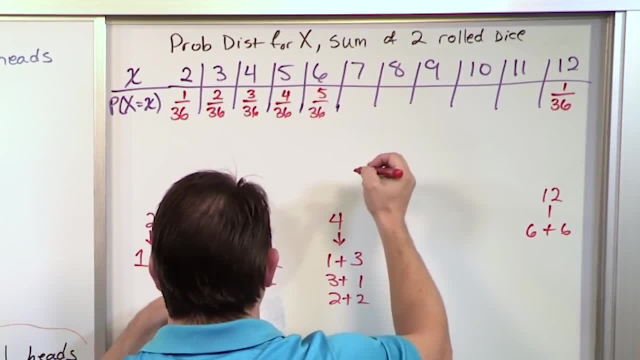 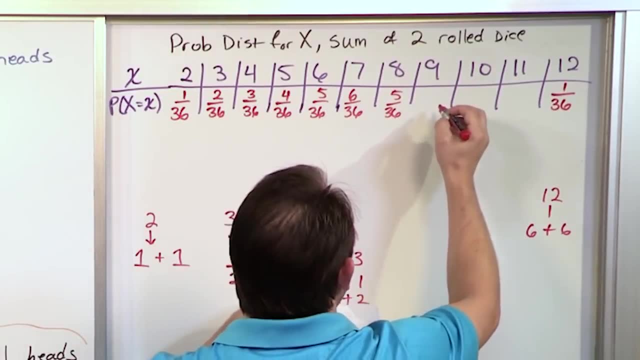 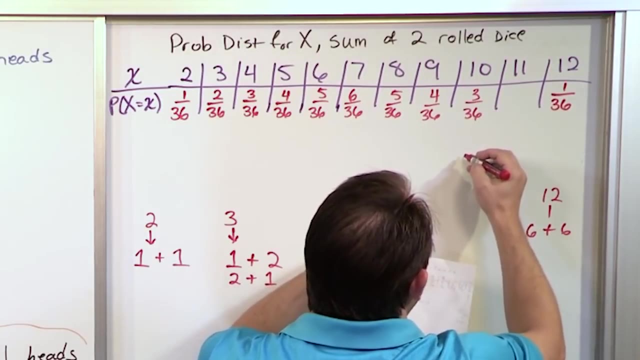 is five ways in which it can happen. This one here is six ways in which it can happen. The number eight: there's five ways in which it can happen. The number nine: there's four ways in which it can happen. The number 10 is three ways in which it can happen. And. 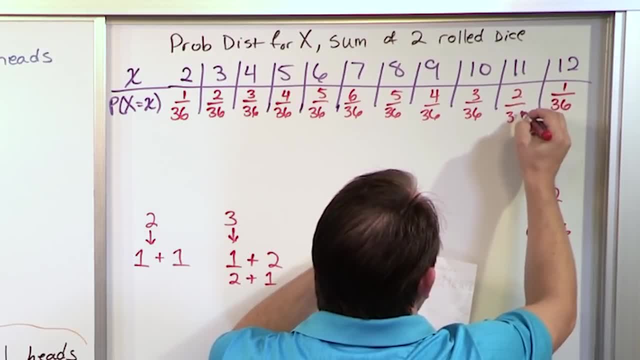 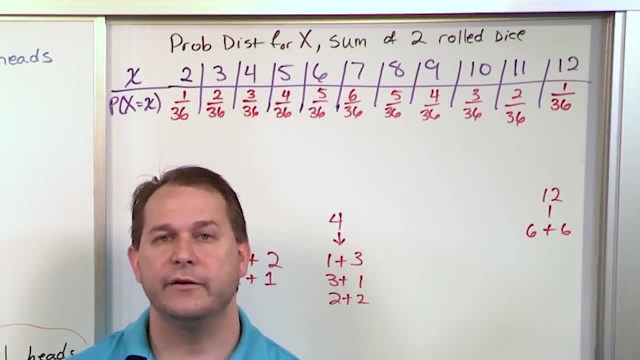 the number 11 is two ways in which it can happen. This one's pretty easy to understand: 11.. The only way I can add to 11 is five plus six or six plus five. There's only two ways in which that can happen, so there's two outcomes. 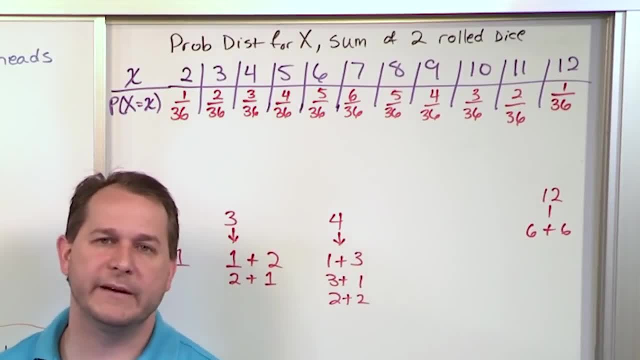 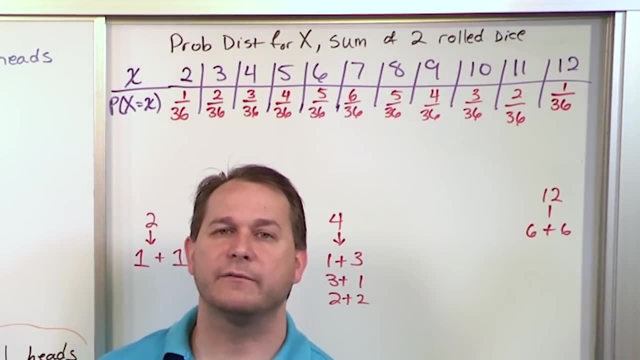 Notice the denominator is always 36, because when we're doing probability, we're trying to calculate how many ways in which my outcome can happen. divided by or with fraction bar over how many possible outcomes are there, There's always 36 outcomes. So now I can look. 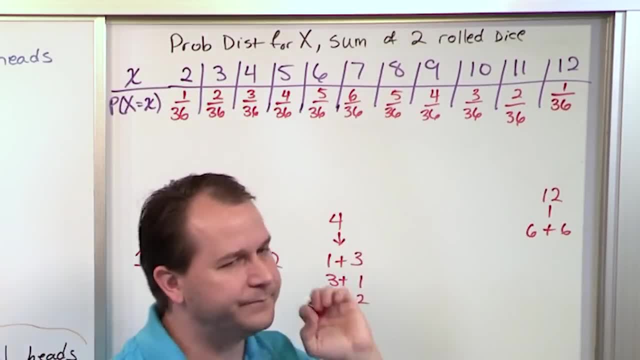 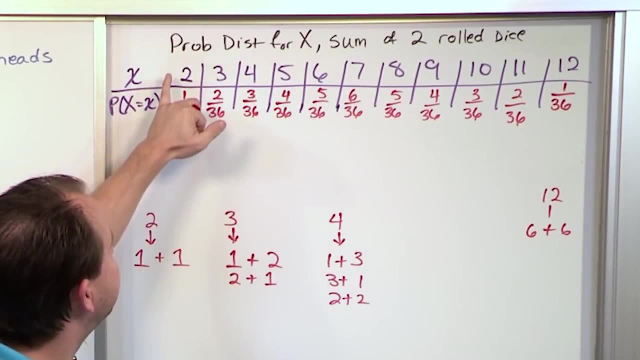 at this. This is a discrete probability distribution. This would be the answer. The reason it's discrete is because my experiment can only end by getting one of these answers. It can only sum to two, three, four, five, six, seven, eight, nine, 10,, 11, or 12.. It can't sum to 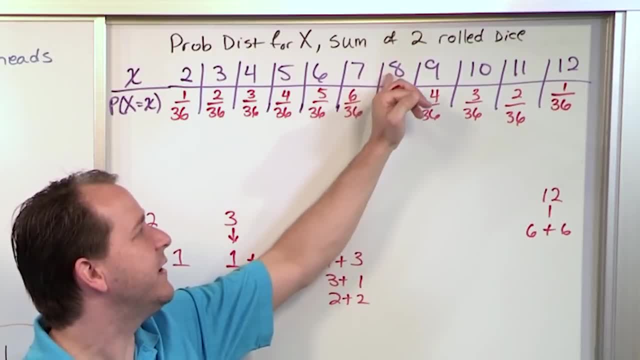 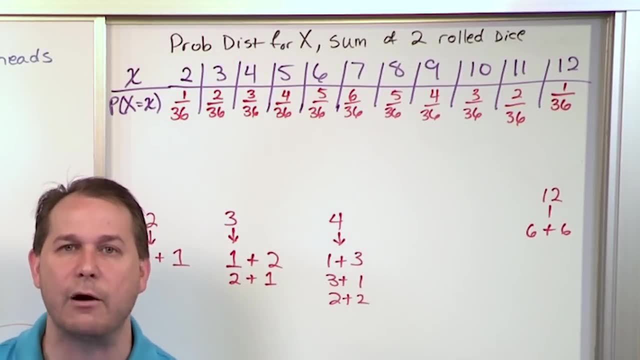 anything else and you can never have values between seven and eight or between 10 and 11.. That could be valid outcomes. You just can't because this is a discrete experiment with a discrete outcome, as opposed to continuous outcomes, like we discussed earlier with heights. 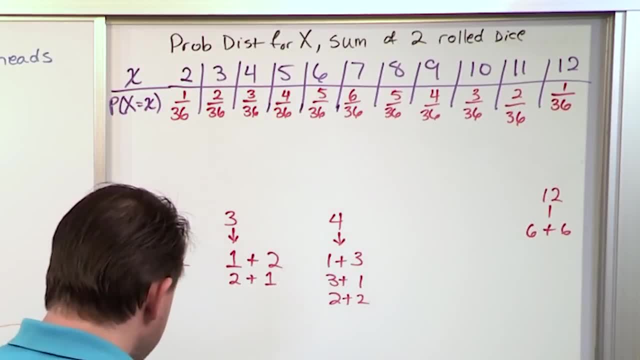 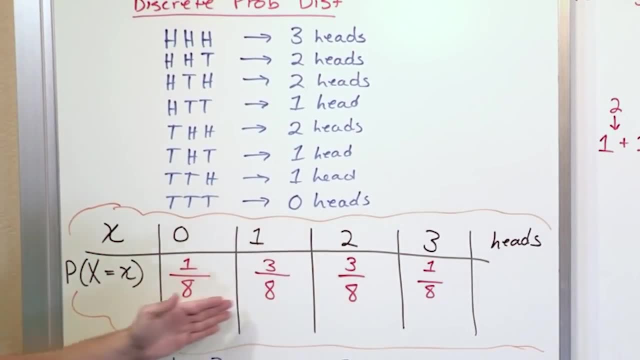 of people and things like that. We'll get to those a little bit later. So this would be the answer. And again, I think I showed you over here. when we talked about this probability distribution, I said the sum of these always have to add to be. 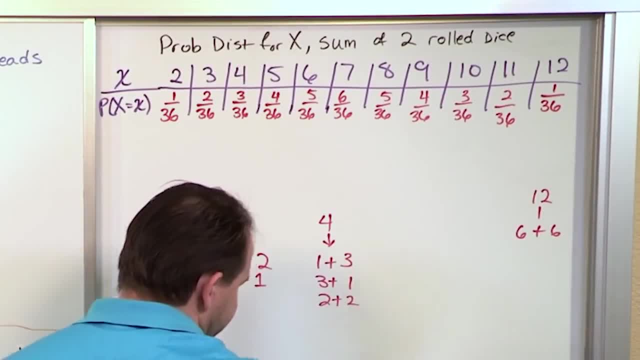 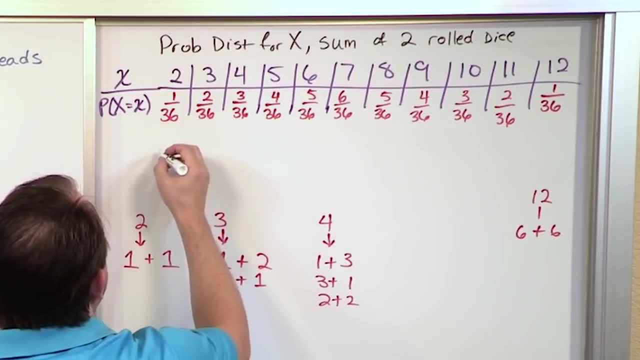 equal to one. Well, the sum of these should always add to be one as well. And if you think about it, all I'm going to do is I'm going to take the sum of these and I'm going to add all of these together. So if I wanted to add, I could say: well, the sum is going. 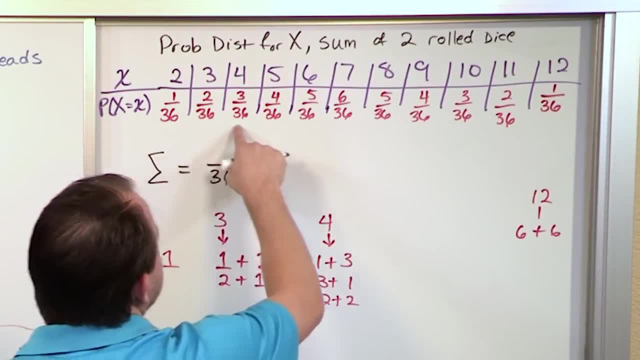 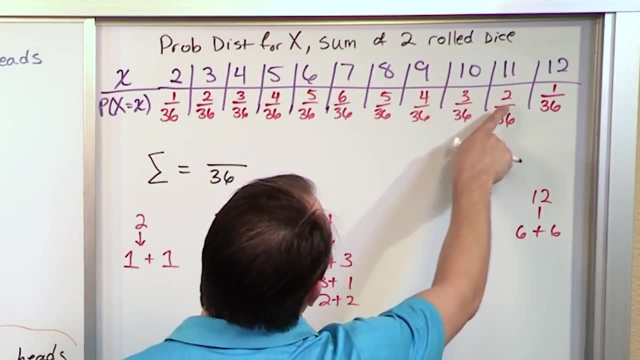 to be equal to something over 36, because 36 is the common denominator. So then I have to add 1 plus 2 plus 3 plus 4 plus 5 plus 6 plus 5 plus 4 plus 3 plus 2 plus 1.. I promise. 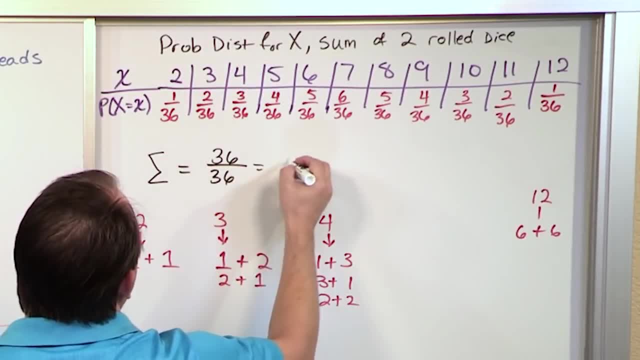 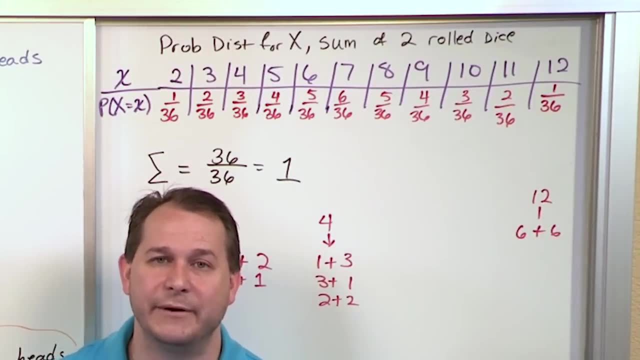 you. if you add that together, you will get 36,, which will equal 1.. That means the sum of all of the outcomes of the experiment have to give you 100% chance of happening. So if I do this experiment, I'm covered by every single possible outcome, because there's no 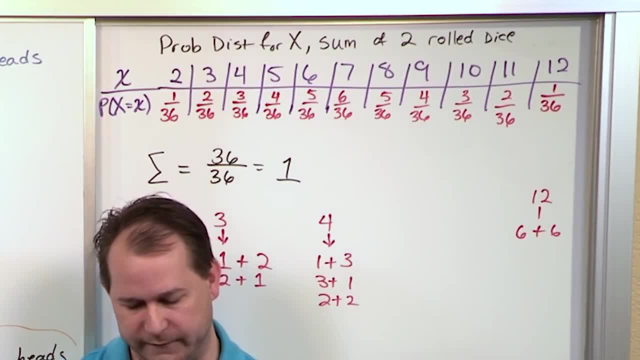 other outcomes there, And so if I add them all together, I should be covered by all of them. There's one final thing I'll show you. here We're getting the probability of each possible outcome of our random variable. We're also showing that we sum all of these things together. 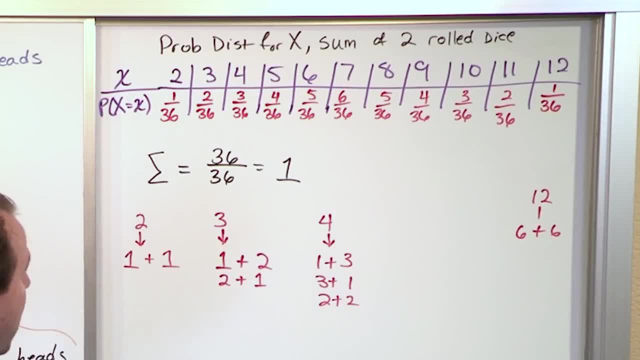 and we're covered because the outcome of all of those sums is 1 or 100%. The other thing is- and we'll get to this a little bit later- if I asked you what would be the probability of getting a sum that is less than or equal to 3? If I asked you that, if I said normally, 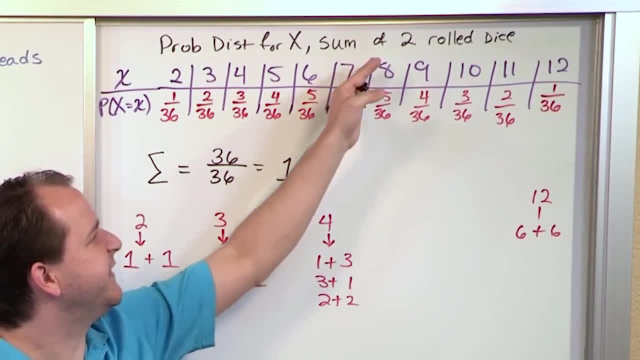 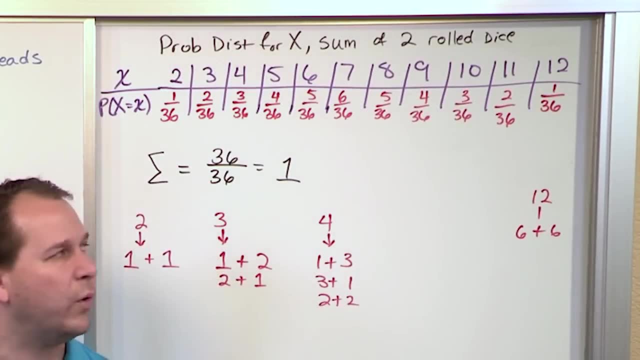 when I'm asking you a question on a table like this, I'm saying: hey, what's the probability of getting a 7 when you sum them together? and you get a 7?? What's the probability of getting a 10 if you sum them together? What's the probability of getting a 12 if you sum? 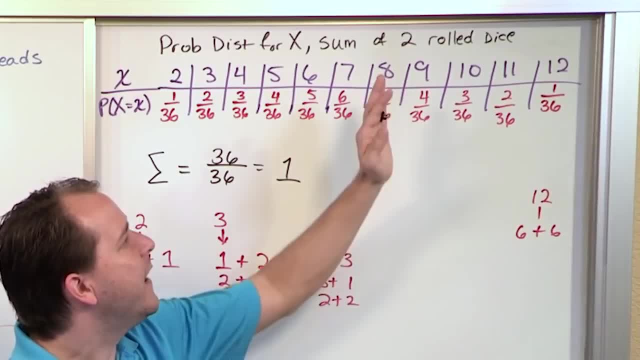 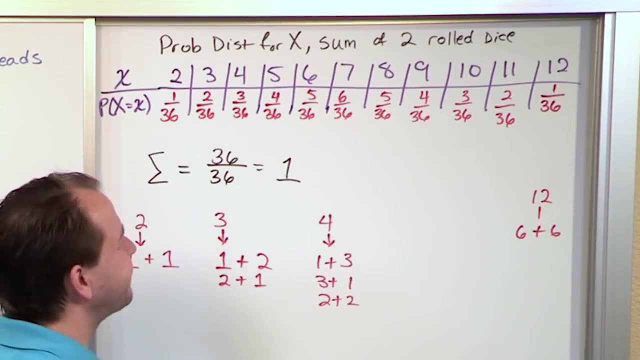 them together. But I can also ask things like: hey, what's the probability of getting a sum less than or equal to 9?? Or a sum less than or equal to 5?? Let's say that we sum all of these things together. Let's say, if I wanted to ask you what's the sum or what's the? 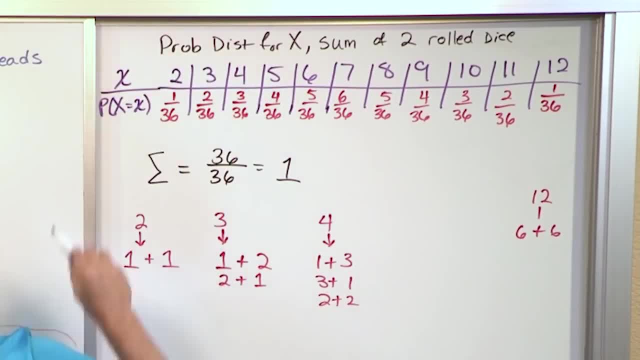 probability of getting a sum less than or equal to 3? That would mean it would be OK if I get a 3 as a sum or a 2 as a sum. So I could say the probability of getting less than or equal to 3 would be the probability of this plus the probability of this, which. 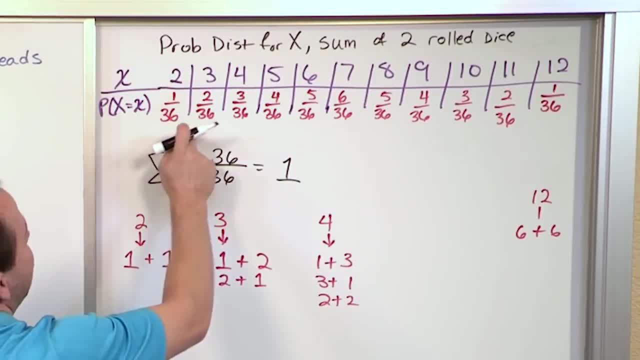 would be 3 over 36.. I would just add the probabilities together. So if I wanted to say, hey, what's the probability of getting a 7?, A 6 or fewer, or a 6 or lower sum, then it would be here all the way down. I would just 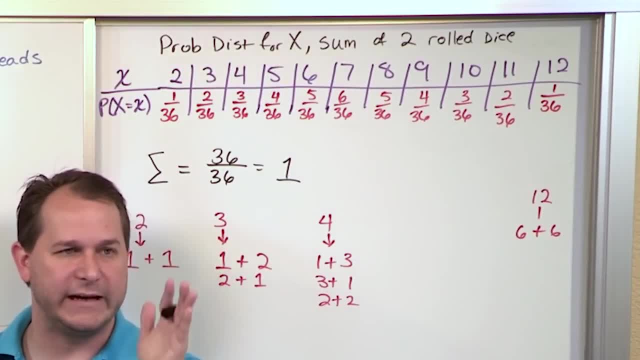 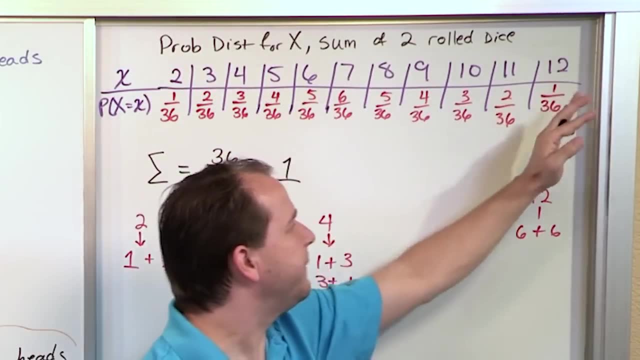 add all of these probabilities together. So, looking at a table like this, you can look at individual outcomes and see the probability. You can also quickly calculate the probability of getting less than something or greater than something just by summing the probabilities of the outcomes together, And we're going to do a little bit more of that later. 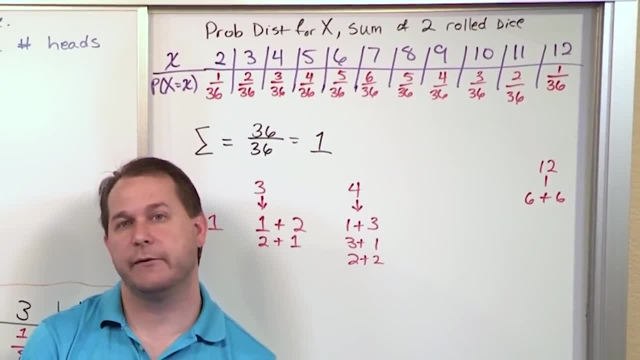 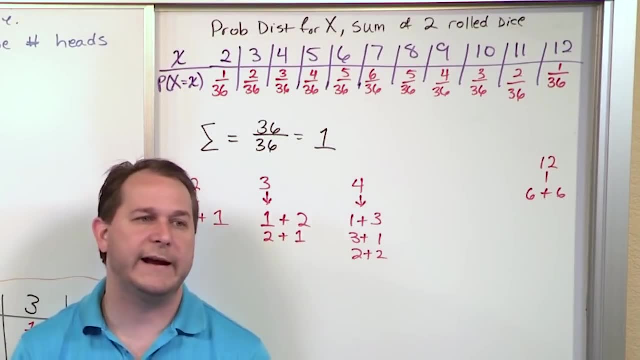 This has turned into a lengthy lesson. I'm going to stop it here. We've covered everything we wanted to cover, But it's so important because the rest of the course is very, very, very important. So this is really going to be built upon doing probability distributions and understanding. 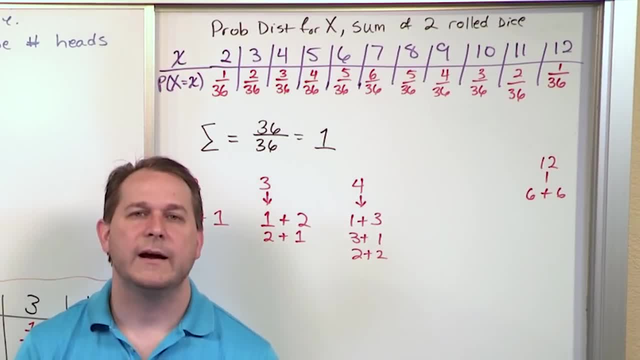 different kinds of distributions And we'll see as we get a little bit farther the details involved in that. But basically you have to understand, backwards and forwards, what a probability distribution is And I hope I've explained that here with a couple of examples. So this knowledge and this kind of mental image that you built of what a distribution, 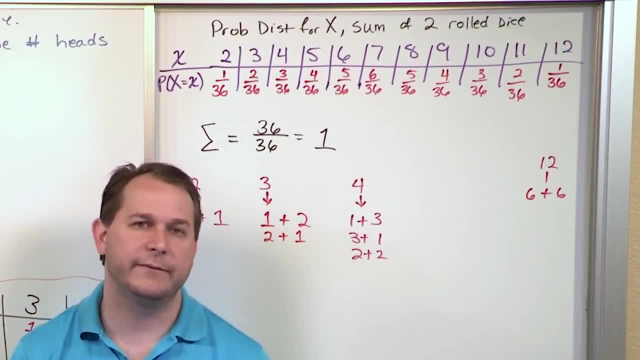 is of probabilities, will carry on as we do all of the different kinds of problems forward. So kind of ingrain this in your head, Make sure you understand these concepts. Follow me on to the next lesson, where we will continue working with statistics and distributions. 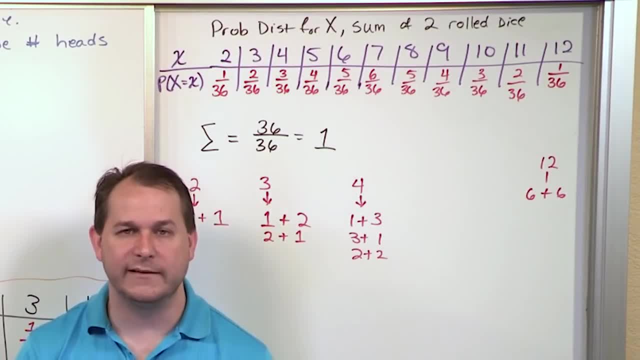 and using those concepts to calculate useful quantities in statistics.